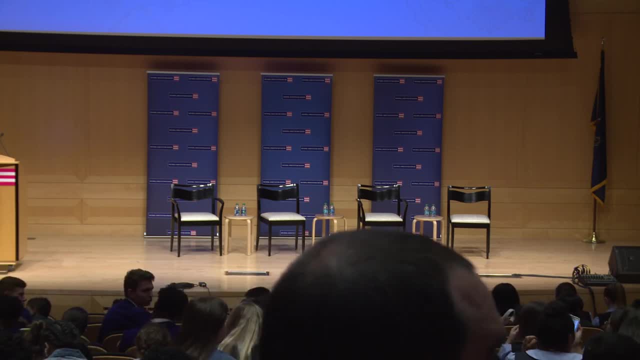 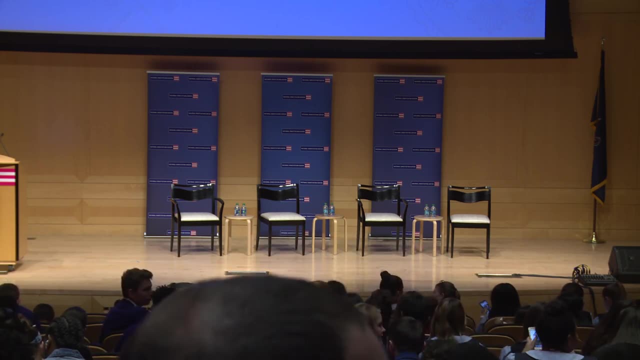 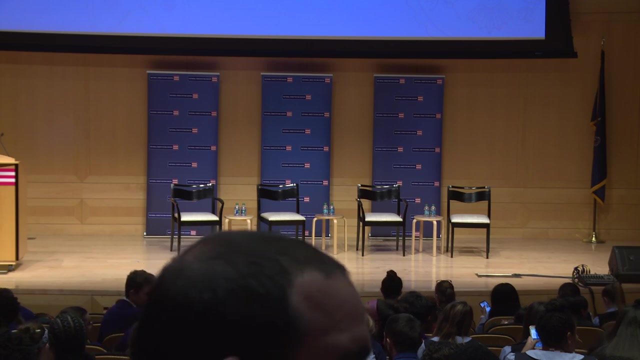 And it wasn't even the point. but she introduced a video and then people were here for a whole different reason and then they started applauding and then they got back to it. Okay, here we go, Let's have fun. That's not very polite, but it's pretty good anyway. 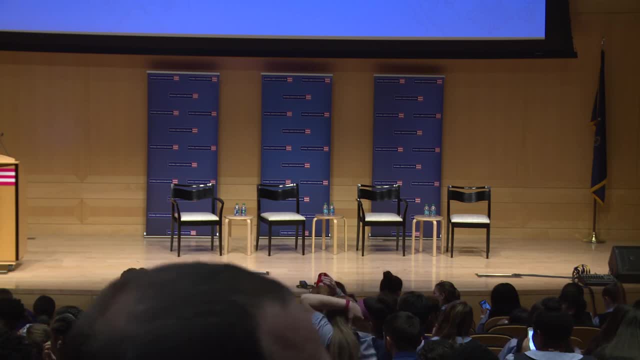 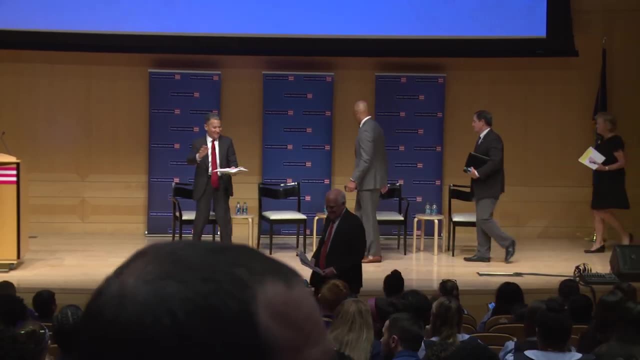 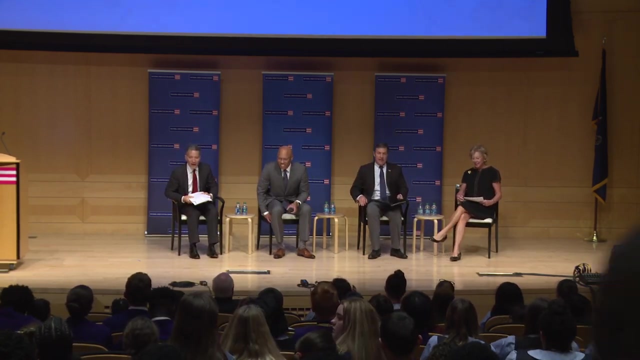 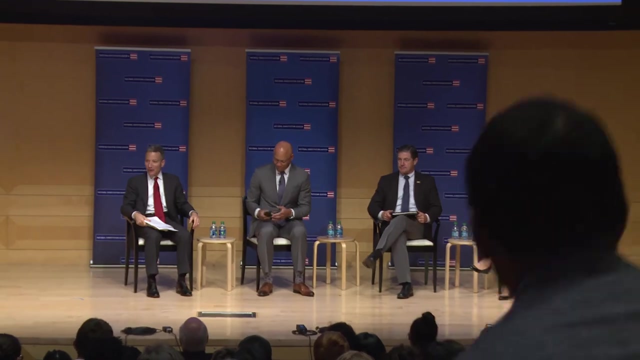 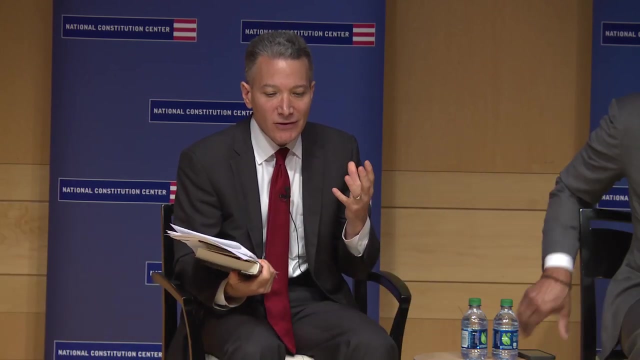 Screwed it up already. All right, thank you, Hi, everyone. Okay, here we go. Good morning everyone. Happy Constitution Day. It is so exciting to welcome you to the National Constitution Center to celebrate this meaningful anniversary of the US Constitution and to talk with you about one of the most important. 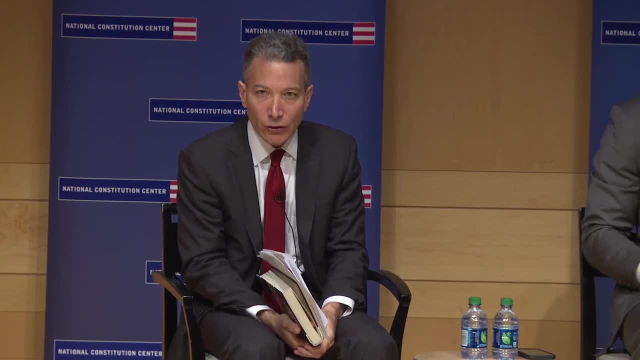 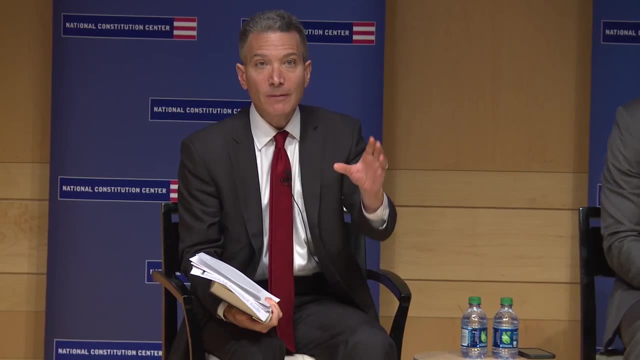 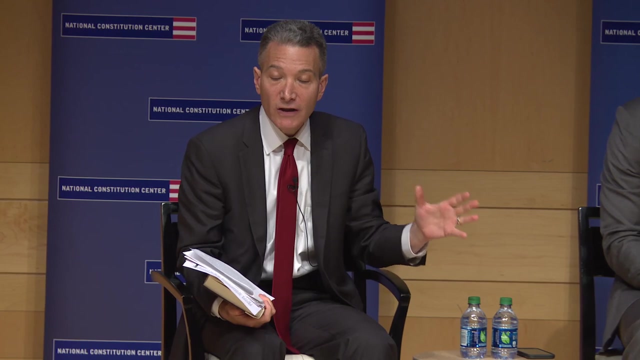 questions in America today. That's: how can we learn about the Constitution? How, as students and teachers, can we inspire each other to learn about it? And then, how can we be ambassadors to the rest of the country to bring our learning across America? I have here next to me America's. 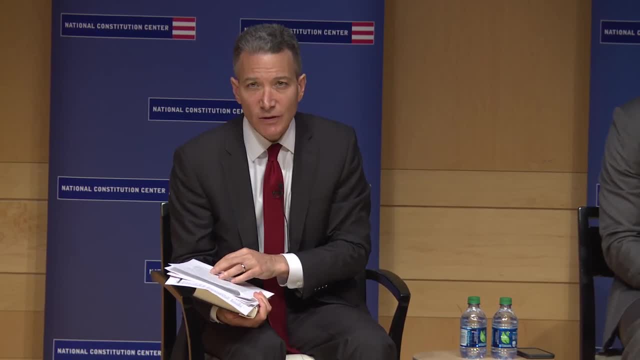 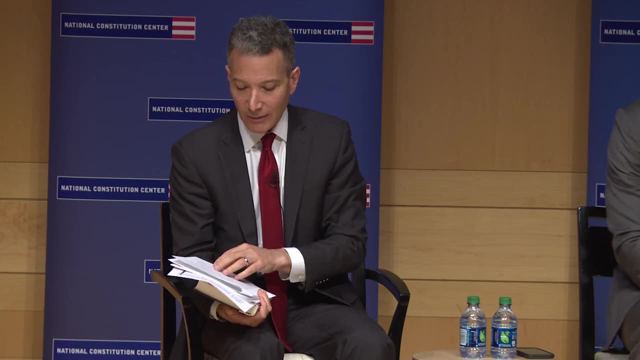 leading advocates for civic education who are doing such important work here in Pennsylvania and around the country. I'm going to introduce them to you and then I'm going to talk to you about some of the most important questions in America today. Thank you. 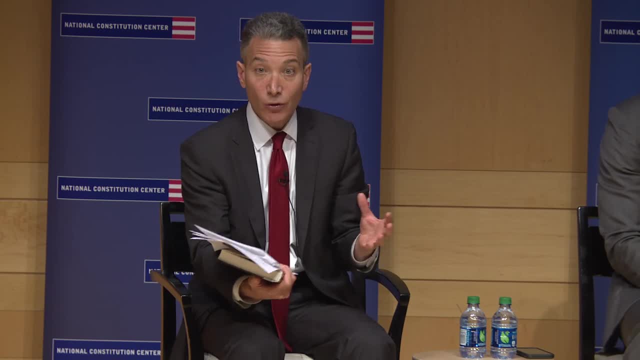 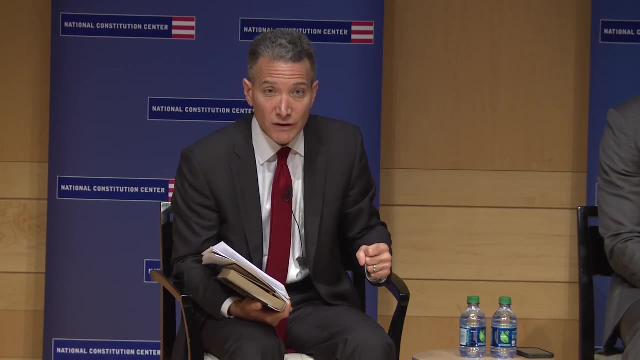 We're going to have some really exciting programs. The National Constitution Center is launched, and then we're going to have a great discussion. So Dr William Hite is the superintendent of the School District of Philadelphia. Let's give him a big round. 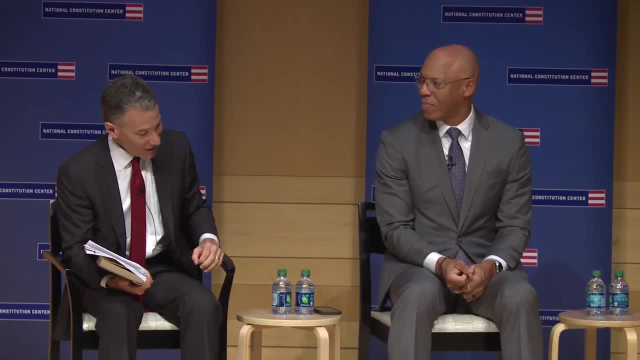 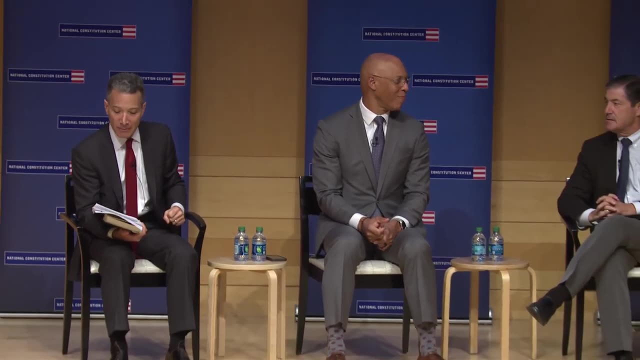 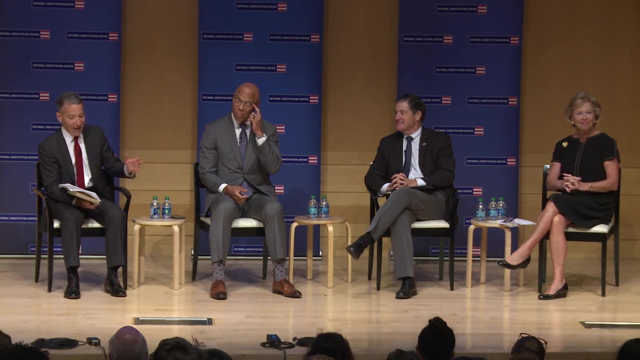 of applause. Representative Jim Gerlach is a former US representative for Pennsylvania's 6th District and a member of the Pennsylvania Civics Coalition, And Judge Marjorie Rendell is senior judge on the US Court of Appeals for the Third. 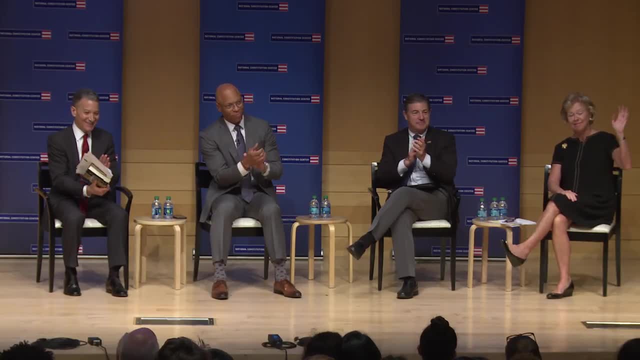 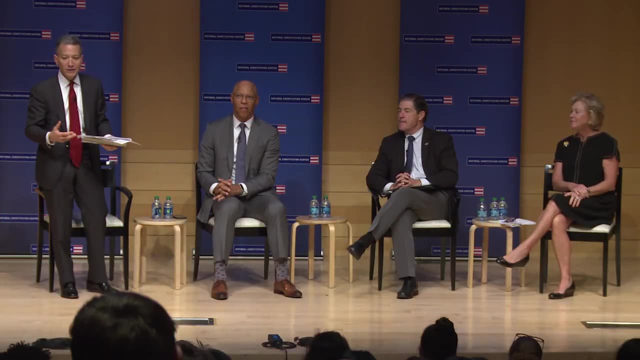 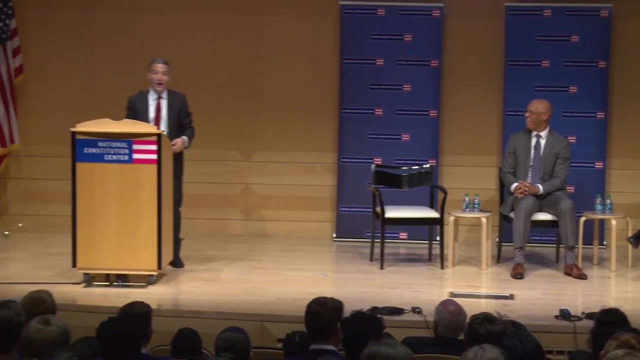 Circuit and head of the Rendell Center. I can't wait to introduce them to you and to have a conversation with them about civics. but now I'm leaping out of my seat because I'm so excited to show you this incredible new online tool that the Constitution Center launched just this morning. It's called the. 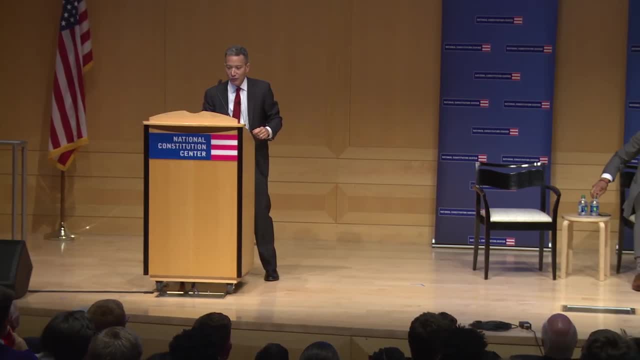 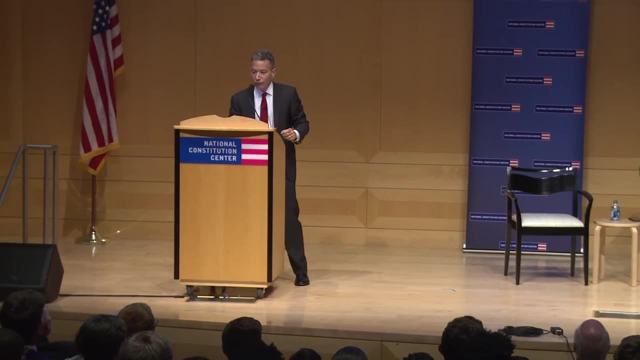 Interactive Constitution Classroom Edition. It's a tool that allows you to learn about the Constitution. You can get it on your on the web for free. You can get it on your iPhones- not now because I'm talking, but after the show- And let's click through Look. 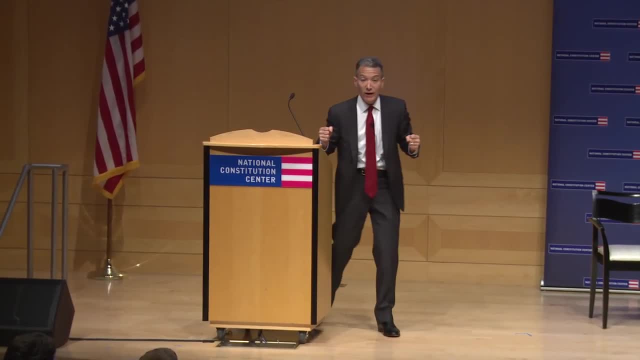 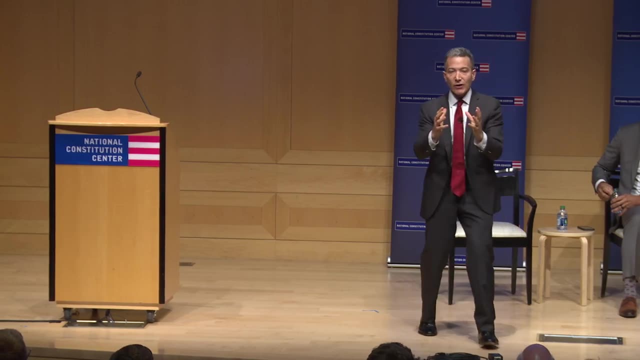 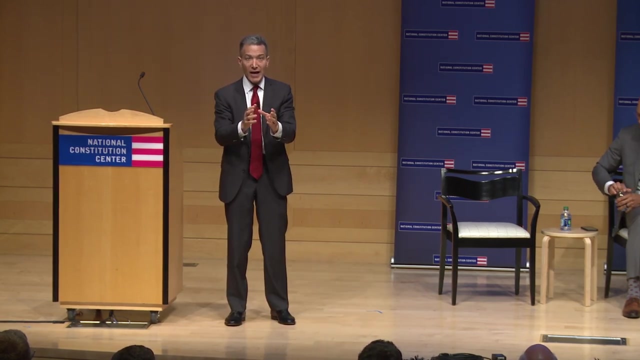 at this amazing upgraded platform. So the original Interactive Constitution was launched in 2015, and it got 25 million hits since it launched And it brings together the top liberal and conservative scholars in America to write about every clause of the Constitution, describing what they agree about and what they disagree about, And it was so popular. 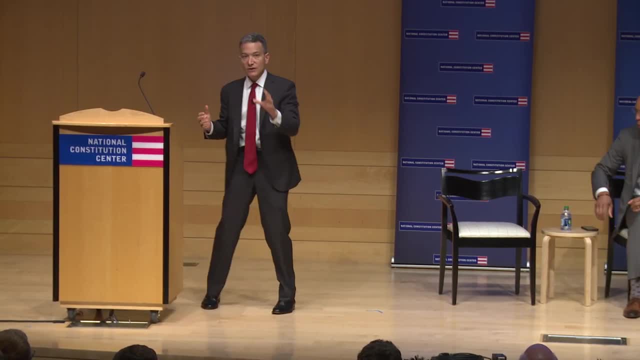 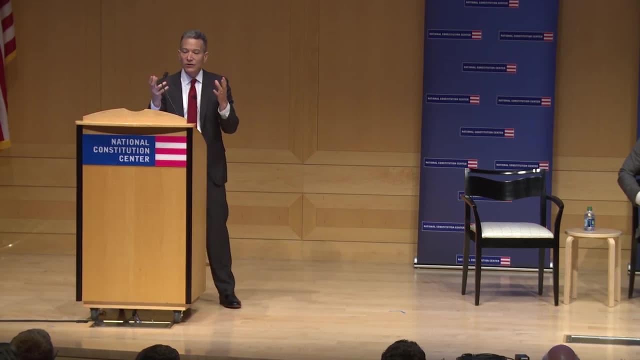 among students and teachers that we created this Classroom Edition so you guys can use it in your classrooms, And I want to show you all of the amazing features it has. And I'm just going to give as an example a current constitutional question. in the news that I 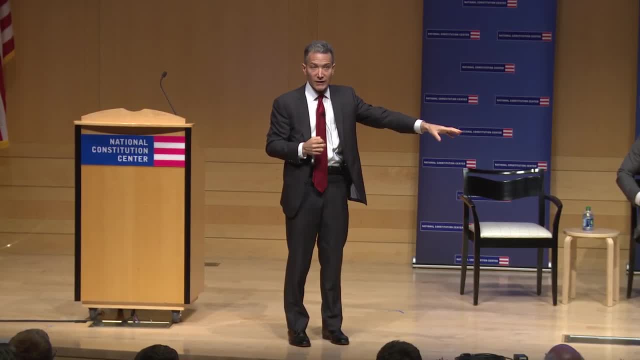 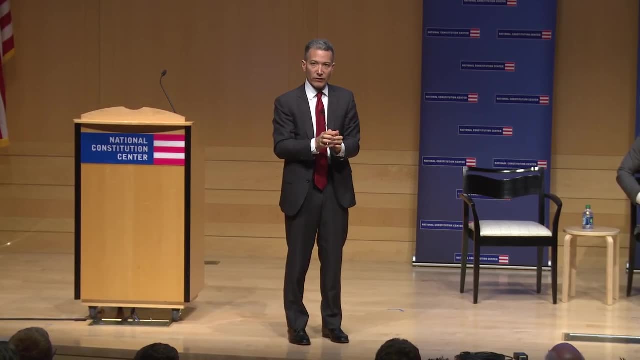 just discussed with a group of students from Central High School downstairs an hour ago. So these great Central High kids came in. We're calling them Constitutional Ambassadors. They're part of a program that we're doing with Dr Height in the school district and 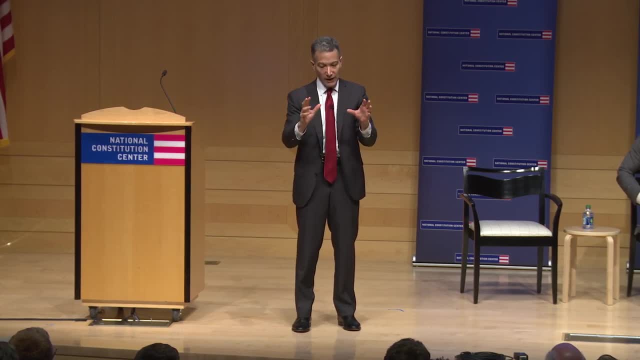 they're trying to bring in tens of thousands of kids throughout the state and the region for an in-person experience here at the National Constitution Center to discuss a constitutional issue. And after you learn about the Constitution here, you'll go back to your classrooms and 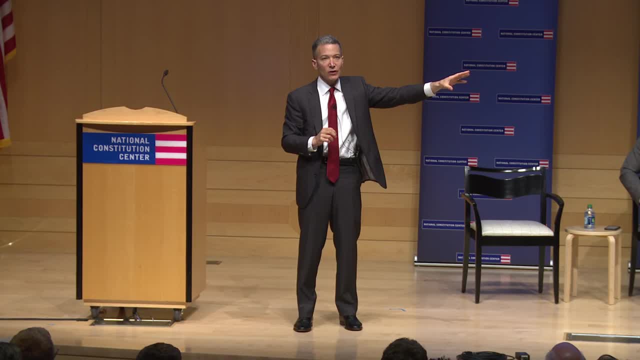 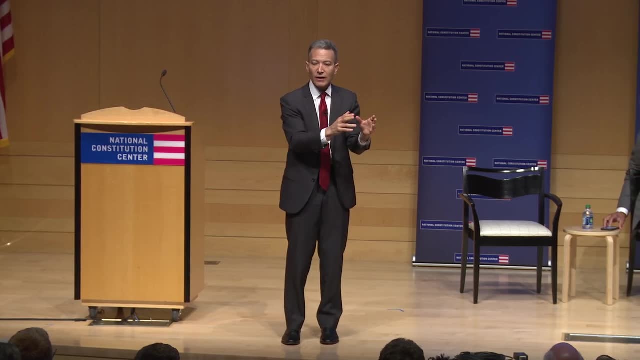 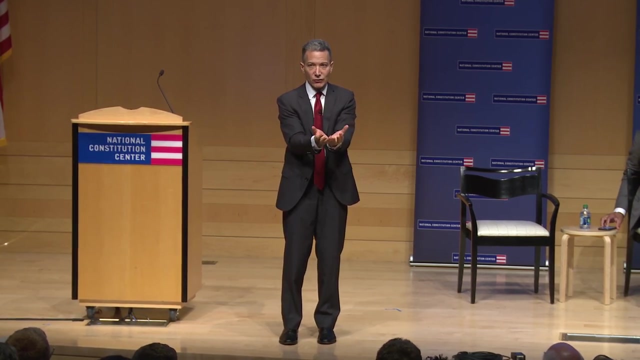 connect with other classrooms across the country on constitutional exchanges. So it is so exciting to see the kids from Philadelphia talking to classrooms from California or classrooms in Ohio talking to those in Minnesota for discussions about the Constitution, modeling it, moderated by judges or master teachers. So the question I discussed with the kids 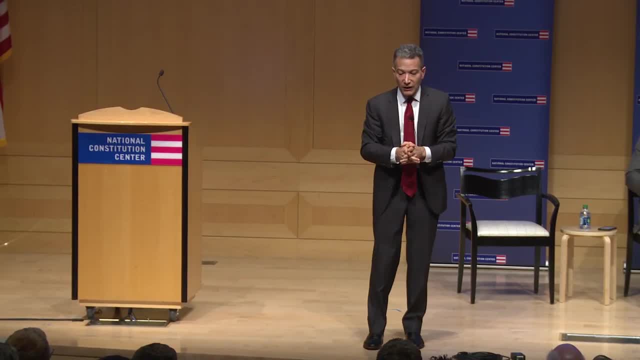 downstairs was a very controversial question, but because we were discussing it in constitutional, not political, terms, we had a very civil dialogue, And that's what I want all of you to do: when you think about constitutional issues, Don't ask what you think the government should do. 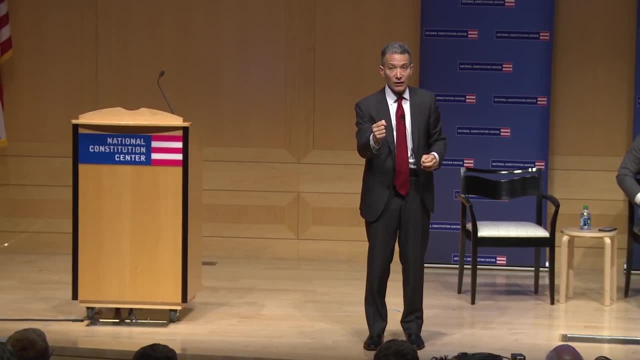 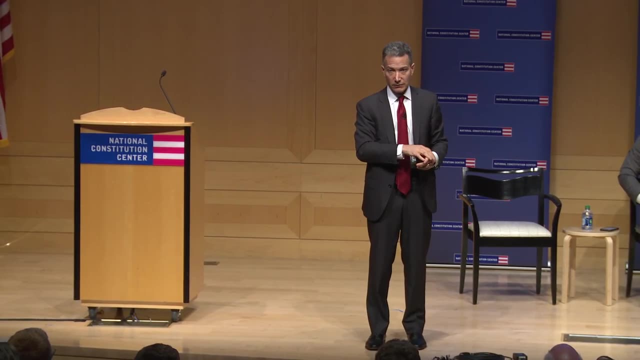 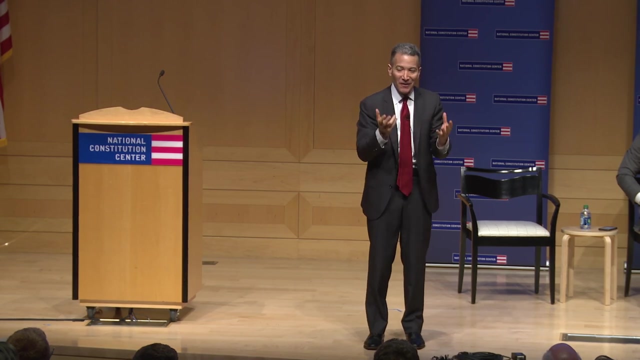 but what the Constitution allows or forbids it to do. And here was the question: Can a public school principal ban a student from wearing the Confederate flag on a backpack? Tough question, It turns out. the lower I saw, you were like whoa, that's a really rough question. 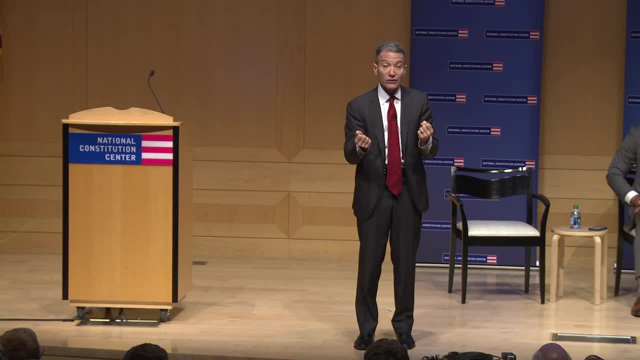 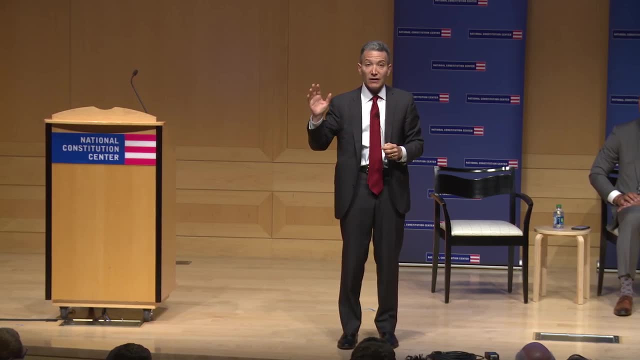 The Supreme Court has not ruled definitively on this question. Lower courts are divided. There are rulings on both sides, so there are good constitutional arguments on both sides. I want to take a quick vote and then I'm going to show you what the interactive. 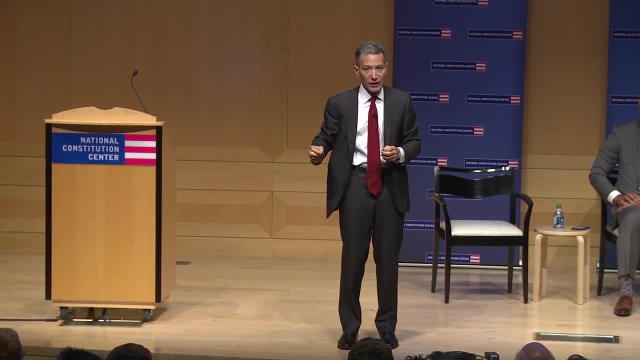 Constitution has. so you can answer a question like that and then we'll vote again, Based on what you know about the First Amendment right now, which says Congress shall make no law. All right, Yeah, there are just one thing we should be really careful about, because I think the Constitution is so tied to the Confederacy, which is beauty and butchering the public school, And the fact that the Constitution does not allow the student to wear a Confederate flag and to wear a Confederate flag, which is not what we meant by a Confederate flag. But the first thing I'd ask is as well, in the case of the Civil War, in the form of the Constitution: do you think that the Constitution allows the public school to ban a student from wearing the Confederate flag on the backpack? Do you think the Constitution does allow the? 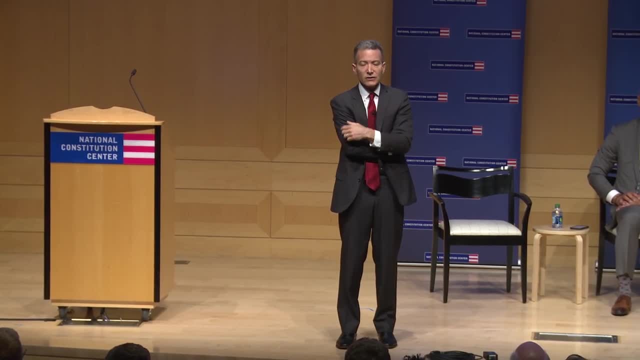 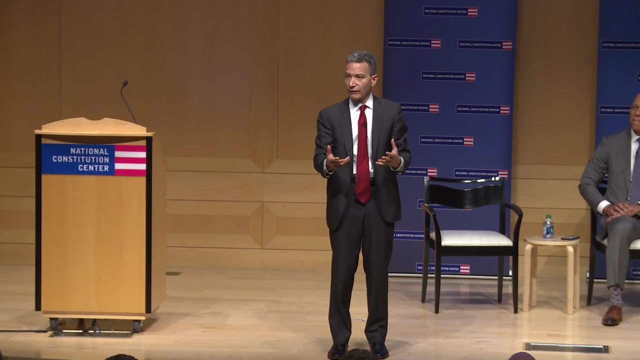 student to be banned from wearing the flag And who thinks the Constitution does not allow the student to be banned from wearing the flag? Most people think that the First Amendment protects the right to wear the flag, And that seems like a really informed vote. 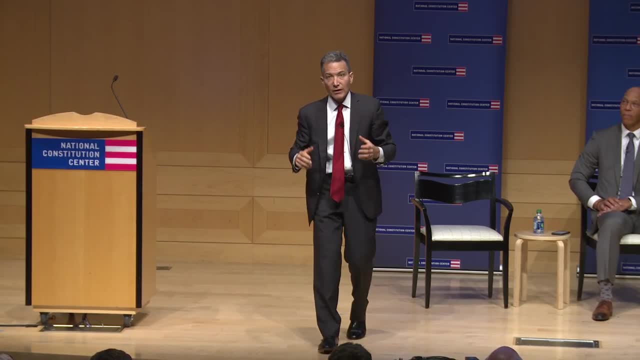 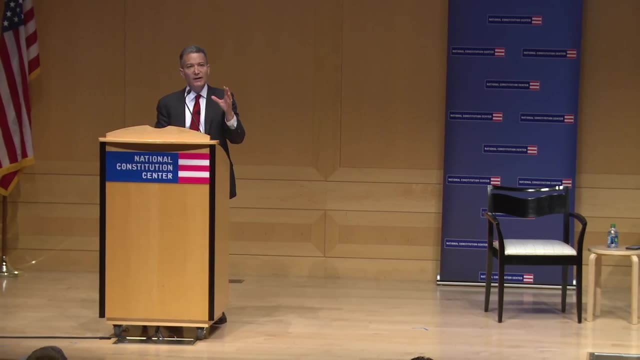 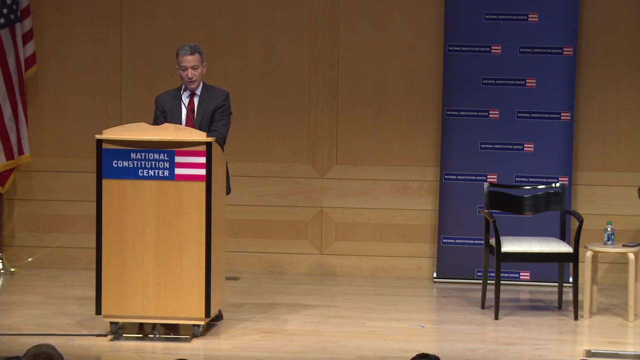 because? Because, as you all know from studying the First Amendment, the First Amendment generally does protect unpopular speech, including hateful and very offensive speech, unless it's intended to and likely to cause imminent violence. That's how strong the test is And you can just see some of the resources. 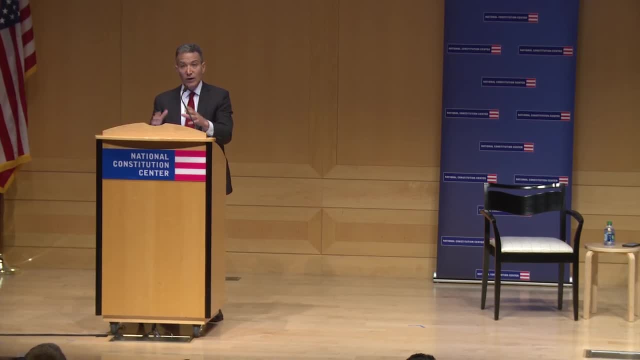 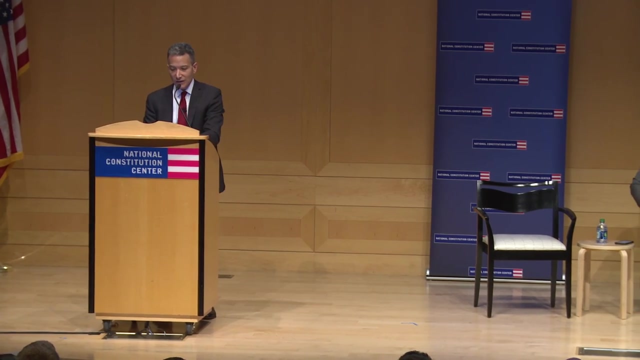 to answer that question here on the interactive Constitution. First you have the experts from both sides discussing what they agree and disagree about what the First Amendment means. Then you have this amazing tool called the drafting table, which allows you to look at the early drafts. 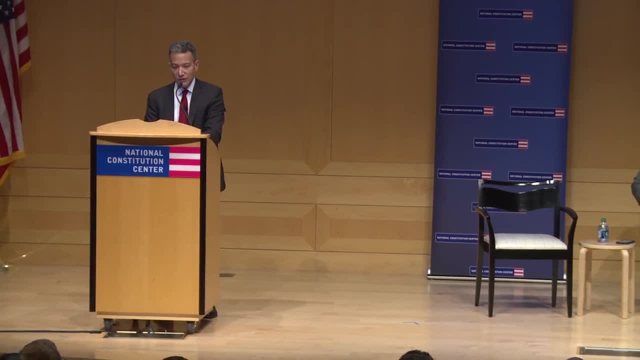 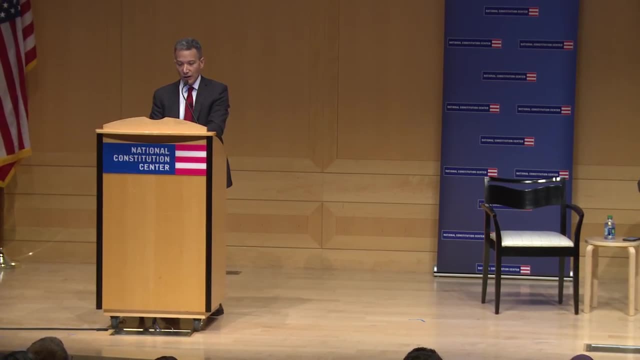 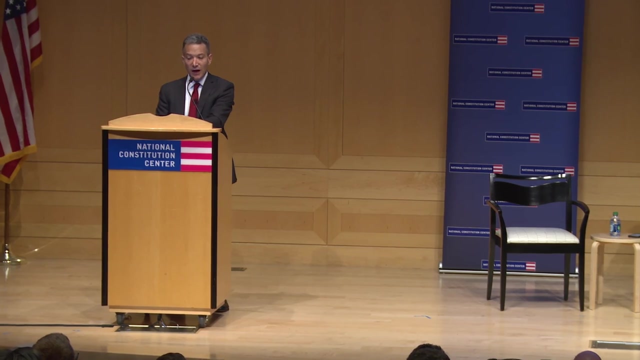 that James Madison relied on when he wrote the Constitution and the Bill of Rights, including early drafts of the First Amendment, which are just remarkable. Then you have this media library with educational videos about the First Amendment, as well as podcasts and blogs about the First Amendment. 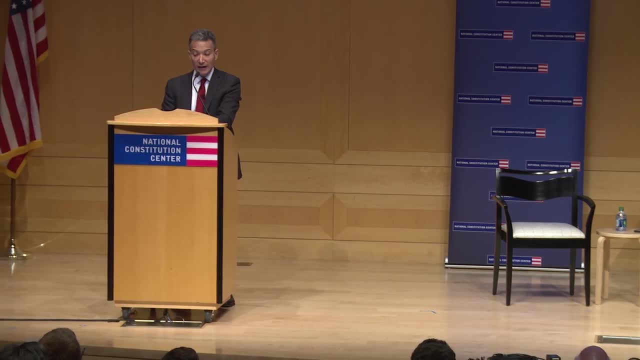 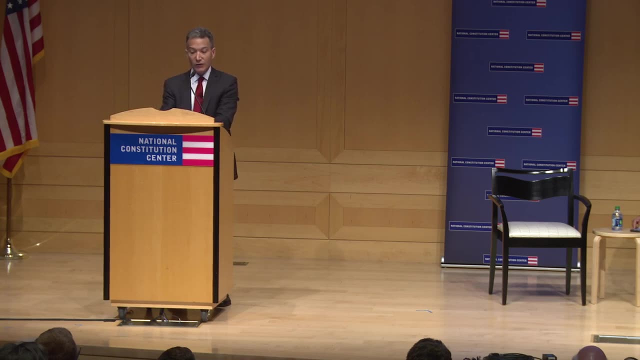 Look at this educational video. We just posted it. It's Justice Elena Kagan who came in and talked to us about what the First Amendment means, And I'm not going to play the whole thing because I don't have the volume. 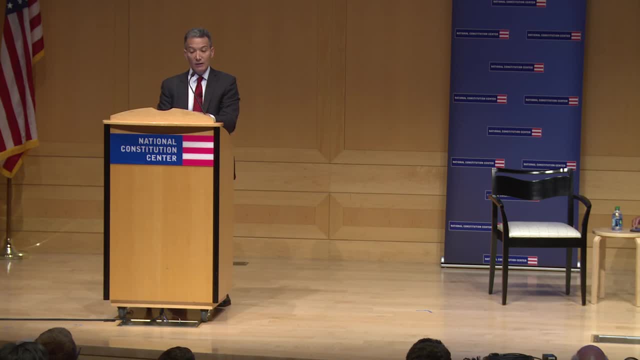 But she's giving us the essence of what she. Why is that in the Constitution at all? Why did the framers put it there? Why they put the First Amendment in the Constitution, And it's so exciting to learn from them. And then the final feature is this Constitution: 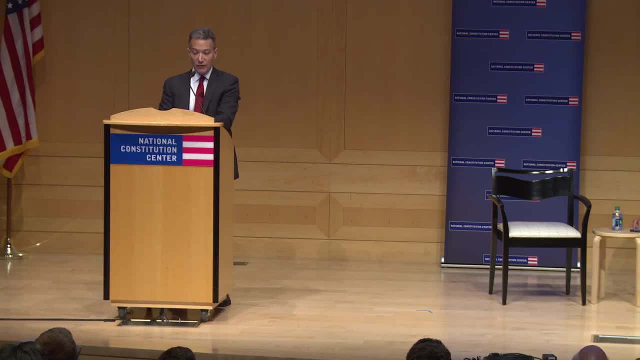 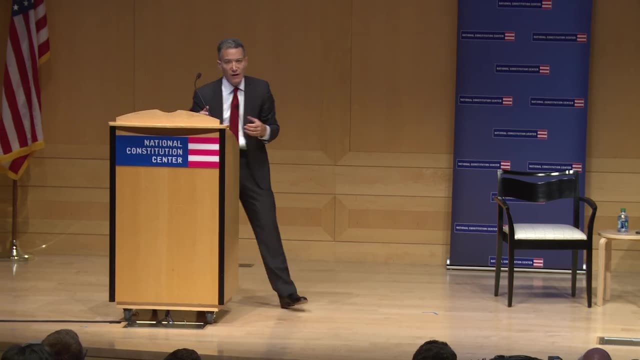 in the classroom where you can sign up for classroom exchanges- There's a wonderful video with Dr Haidt talking about them- And be paired with classrooms across the country for First Amendment discussions. So imagine doing that for all All 80 clauses of the Constitution. 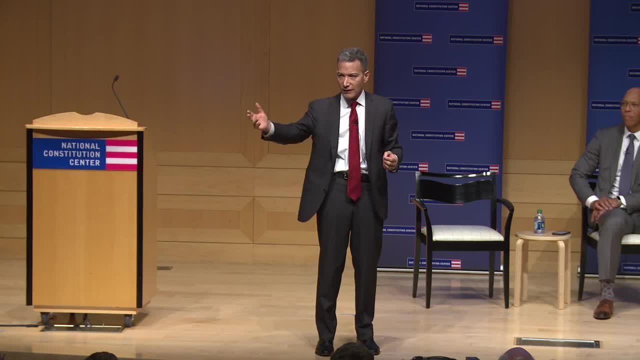 I just showed you the First Amendment, But there are 80 clauses. There's the 27 amendments, There's seven articles. There are lots of individual clauses, like the Commerce Clause or the Export and Port Preference Clause or the Foreign Emoluments Clause. 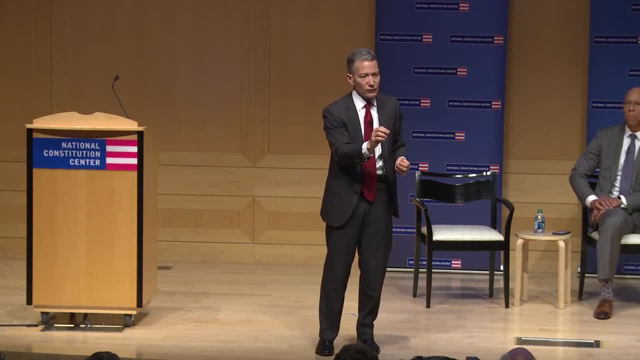 the stuff that's in the news. Think of how much learning there is for each of you to do. I'm a law professor. I learn something every single time I look at this tool. pick a clause I don't know about and dig in deep with the experts, the videos. 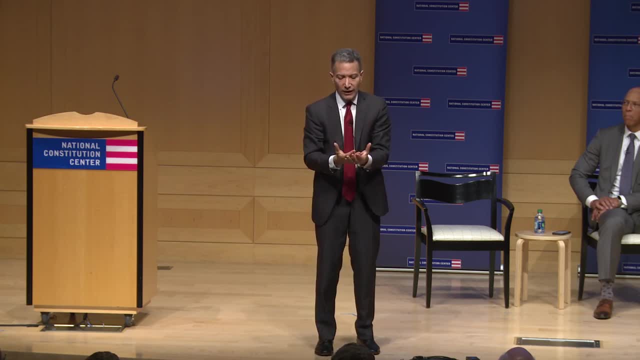 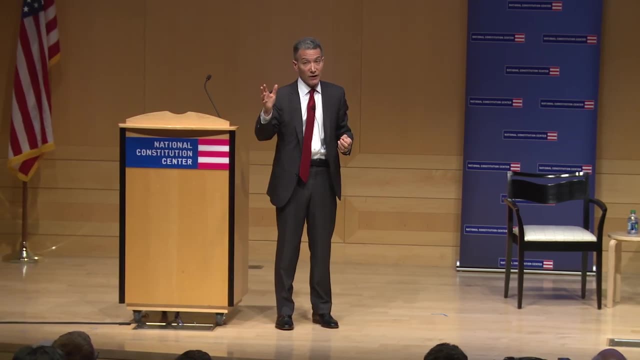 the podcasts, the blogs And the early drafts. It is just a thrill to be able to learn about the Constitution and to show you this tool. OK, I'll just cut to the chase because we've got to begin our discussion. But it turns out that a court in 1972. 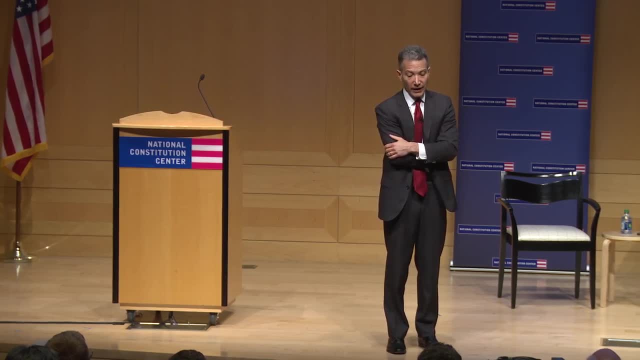 held that a school did have the right to ban the student from wearing the flag, Because, although all of you who voted the other way are correct, that the court held in that case involving the black armband when the student was protesting the Vietnam War, that you're right. 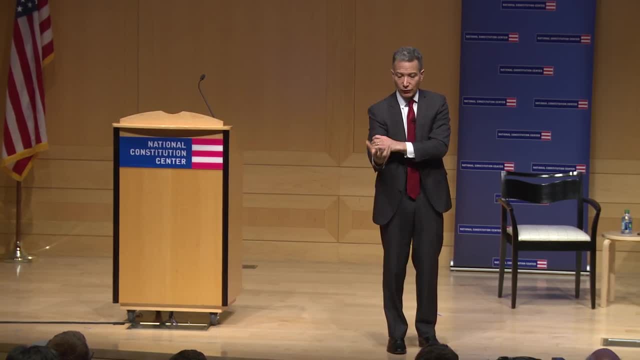 You don't stop at the schoolhouse gate and you generally do have the right to protest government actions as a student. Nevertheless, there was another case that said that if the speech is likely to cause substantial disruption in the school, then it can be restricted. 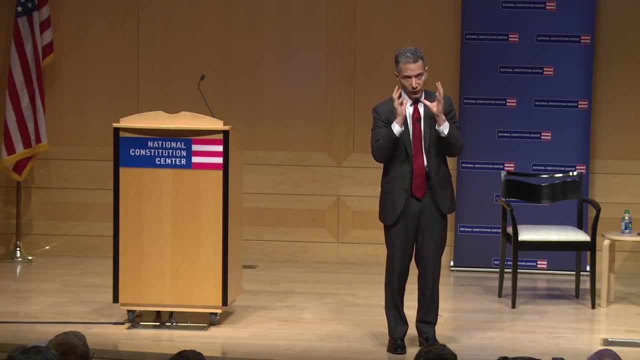 And in 1972 in Georgia that judge held that that Confederate symbol was so explosive that it was likely to cause substantial disruption and could be banned. But other courts have held the other way. So so much to learn, So exciting for you to be among the first students. 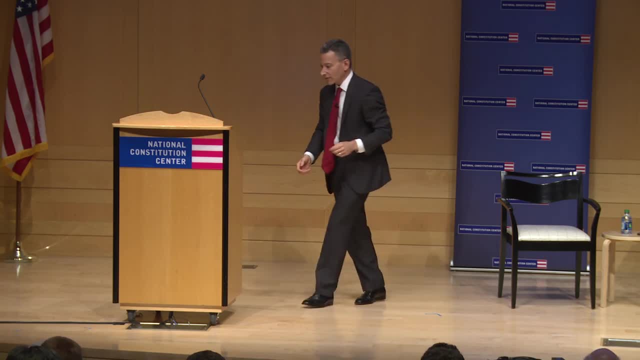 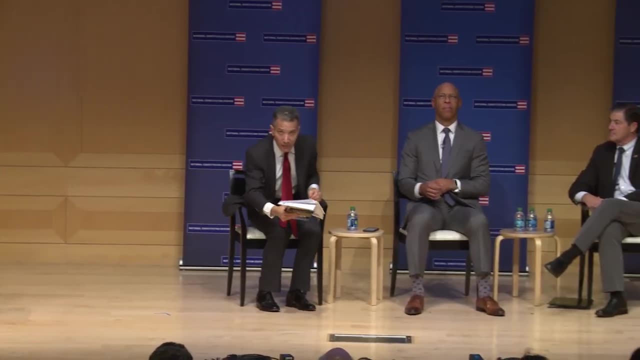 to show this great Constitution, A Constitutional, Interactive Constitution too. I'm going to now pick up my book and introduce my great colleagues, all of whom are doing similarly dynamic work together and by themselves, And they're going to tell it about you now. 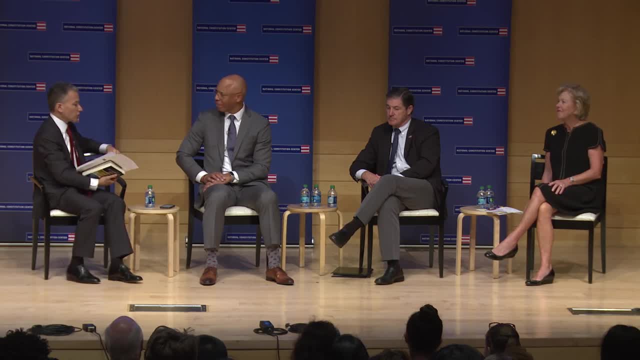 Dr Height, I'm so honored that we are working together on the Constitutional Ambassadors Program, So grateful for your visionary leadership of the school district. Tell the group about what we're hoping to do with the Ambassadors Program and then talk more generally about what. 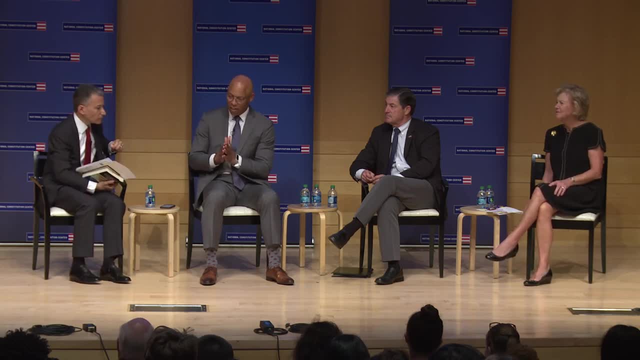 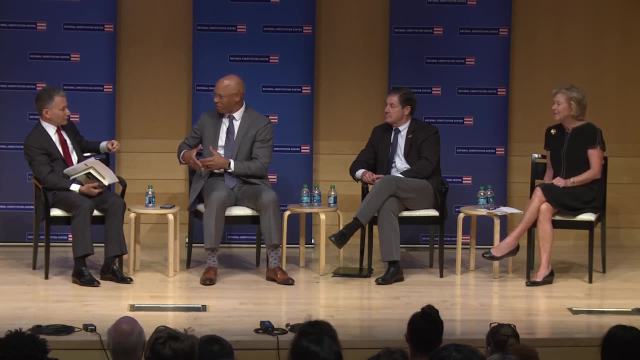 the school district is doing to promote the teaching of civics Great. First I'll talk about the Ambassadors Program, And it's with a partnership with the National Constitution Center, So thank you for working with us on this program. This is a program that allows young people. 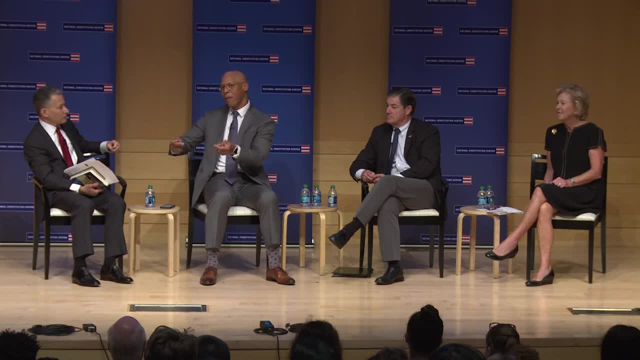 to engage with content, then work with the educators here at the National Constitution Center, either here on site or in their schools, And then, once they do that work and become more knowledgeable, then they can go back to their schools and engage in dialogue with other students at their schools. 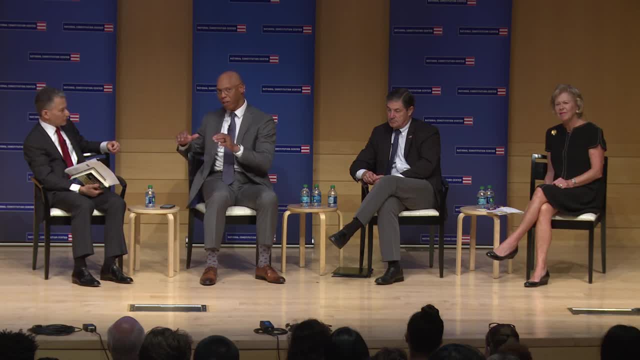 other students in schools across the Commonwealth- the city of Philadelphia, then the Commonwealth of Pennsylvania and then across the country, And so it is a way to have young people participate in the type of civil discourse that you just described, And so we're really excited that we 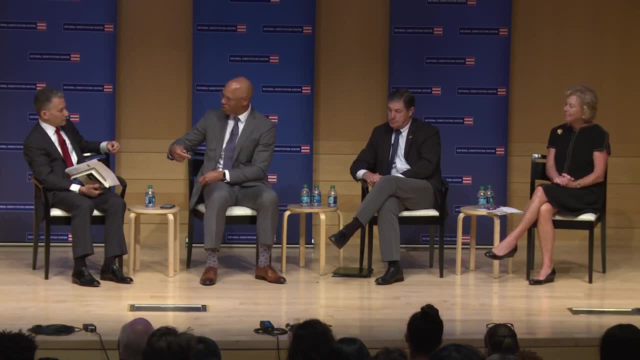 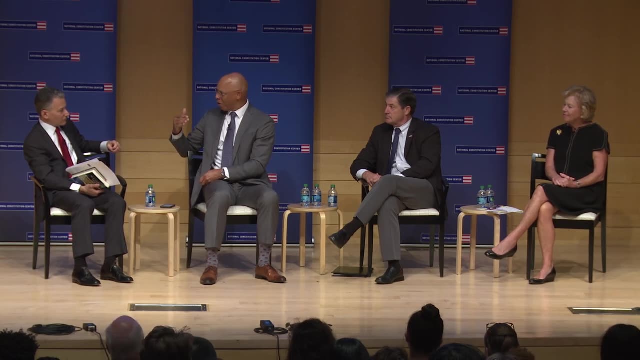 will be a part of the opportunity for young people to be these ambassadors. And here's the other thing that I think is really important: Generally, as our young people go, and when they talk about certain things, then those things also become the things. 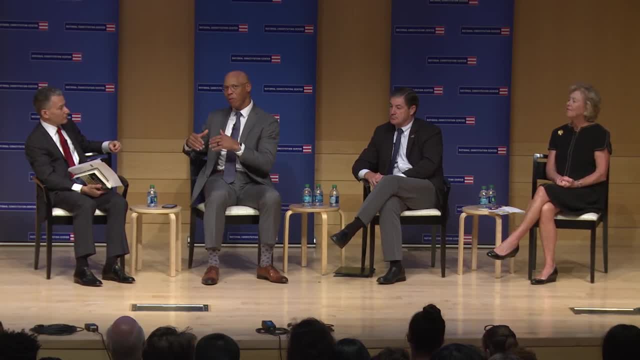 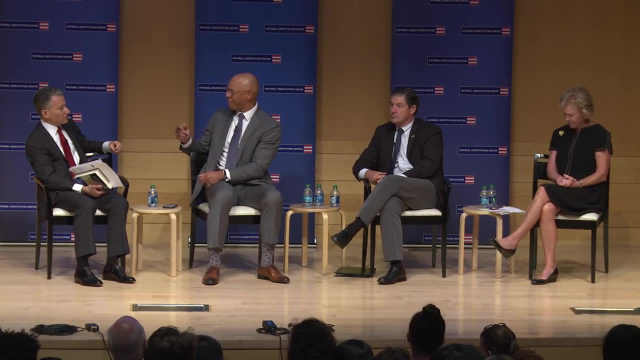 that are talked about in their respective communities, And so if young people are talking about the Constitution in their neighborhoods, in their communities, or just referencing it, it's a good possibility that more individuals will then either look up something with the Constitution, And so this notion of ambassadors becomes more. 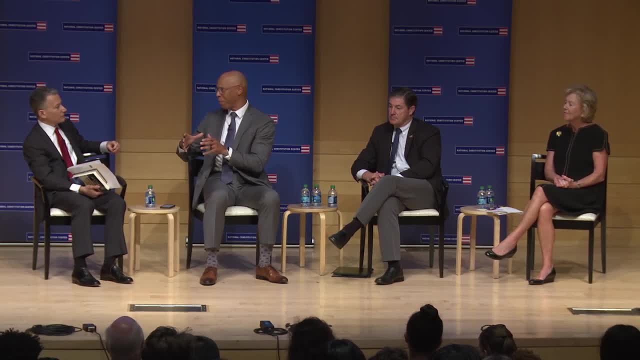 than just young people engaging with other young people, but young people engaging with their communities writ large, and so we're really excited to be a part of that. that's so wonderful. and the school district as a whole is creating a civics test, as Pennsylvania law now requires. tell us about, yeah, so 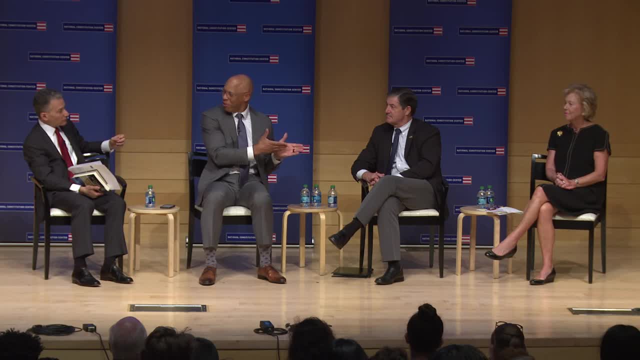 and and thanks to Jim and others, the representative and others who put together act 35, and Act 35 now requires, for between seventh and twelfth grade, an assessment on civics, and in the school district of Philadelphia we have begun preparation for that in two ways. one, we are doing a substantial rewrite of our 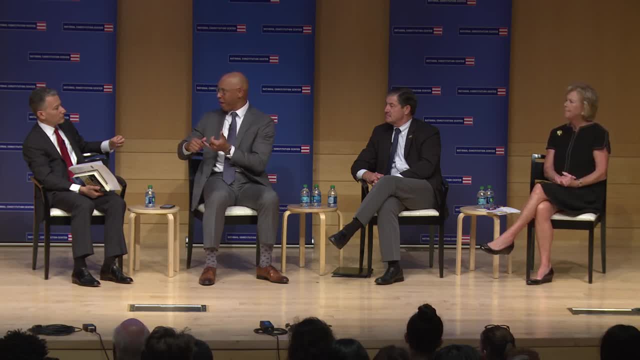 civics related standards in grades four through eight and in US history and and in world history, and we're thinking about ways to also include those conversations as a part of our African American history course and our US history course as well. So we've had development with teachers on this. 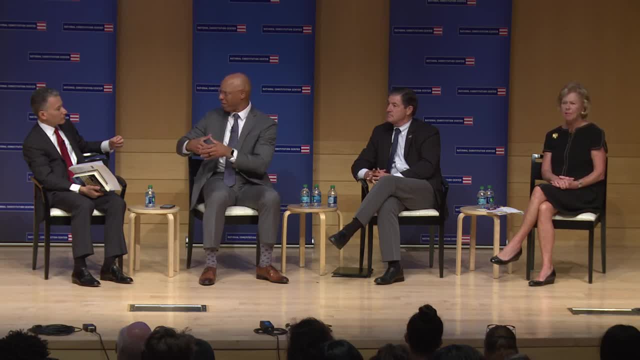 and teachers. we had over 50 teachers come to an event, a development event. they're gonna be a part of that. We've hired an individual who is responsible for writing in the civics curriculum and developing our teachers and this is gonna be informed by many of the teachers. 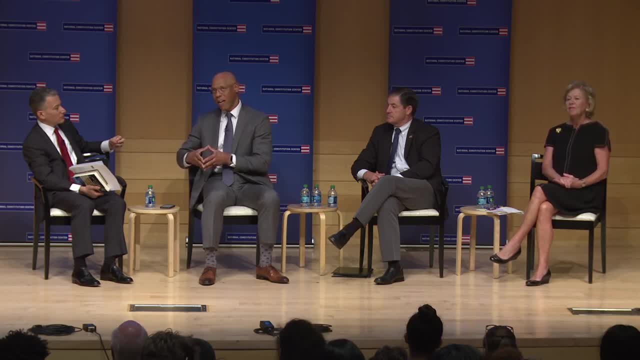 who are working along that process as well. So we hope and are very excited about having this as a part of what our young people experience, not just as their high school experience, but beginning as early as grade four. That is wonderful that we're starting teaching. 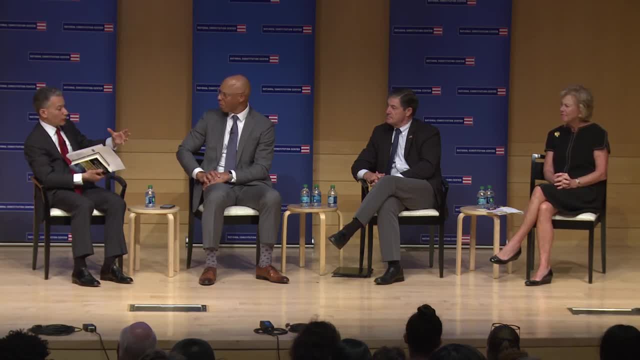 as early as grade four, and it's great that you're developing this and we look forward to working with you as you develop the test and hope that we can integrate some of this interactive constitutional material as well. That's wonderful, Representative Gerlach. 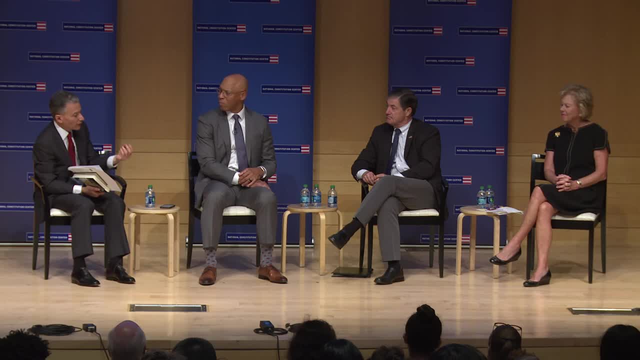 you had the vision to encourage the state of Pennsylvania to adopt this civics requirement. Tell us about the genesis of Act 35, why you think it's important and what your great organization, Pennsylvania Civics Coalition, is doing to help teachers meet it. 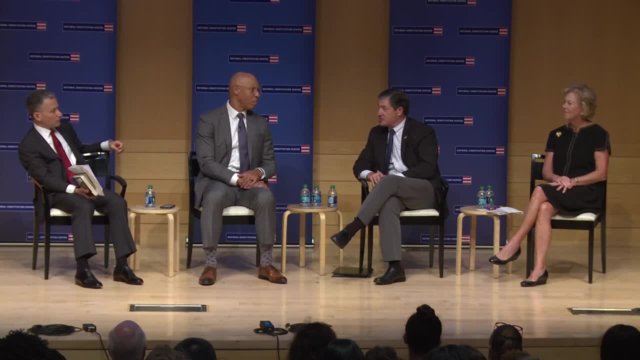 Thank you. Well, civics education's always been an issue before the General Assembly in Harrisburg, at least since I go back to my state legislative days in the early 1990s. but there's never been up until Governor Wolf signing into law Act 35,. 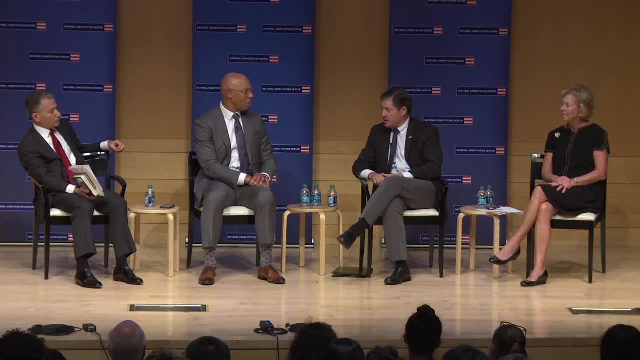 a consensus around what better civics education ought to be in Pennsylvania, But to the credit of the legislators in Harrisburg and Governor Wolf, they did get that enactment passed, and so it does now mandate this test beginning next year for all the school districts around Pennsylvania. 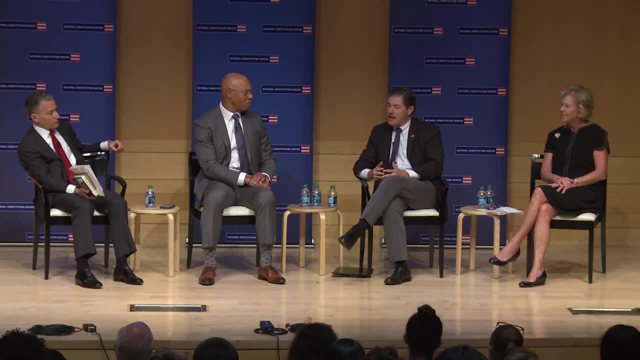 And what sort of coincided with that. at the same time was at the federal level, the former members of Congress Association decided to make civics education an important initiative for our association. So about a year and a half ago the association decided to encourage former members to go back to their states. 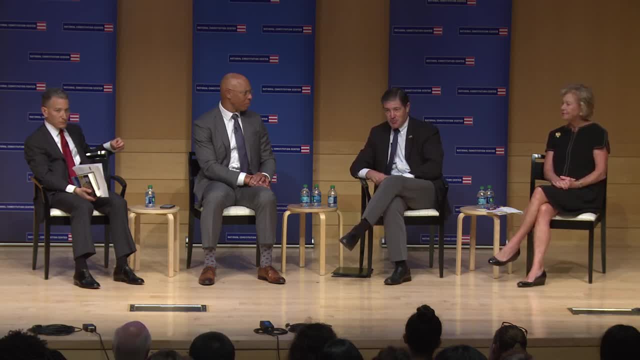 and try to promote civic education. So in Pennsylvania, Congressman Jim Coyne of Bucks County and we have about five Republicans and five Democrats plus a number of other organizations, Glenn Rendell Center that Judge Rendell is so much leading that we want to try to support state government. 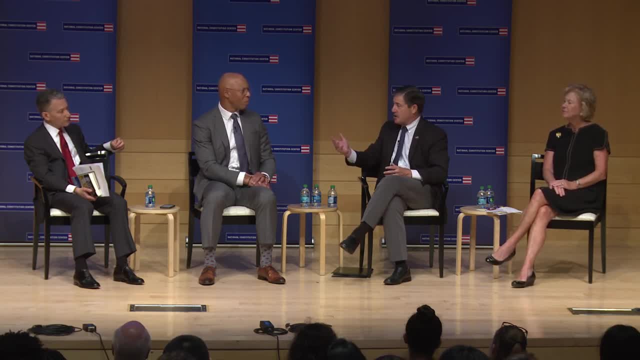 but also all of our teachers and educators around the Commonwealth, including Dr Height, by trying to help develop the resources for implementation of Act 35, by trying to engage in our communities, where our old stomping grounds were as legislators, but other places around the state. 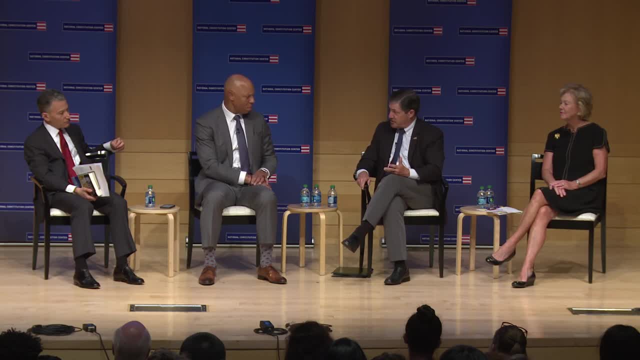 and engage not with just students, not with just educators, but with the communities at large, Because, ultimately, citizenship is everybody's business. And you know, it's been said in the past that great citizens are not born, they are made. 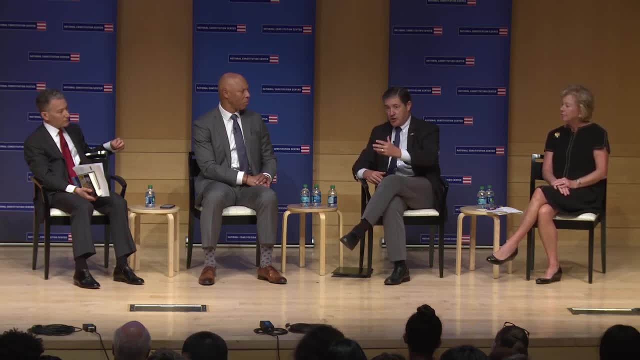 And so, to the extent that we can help in this process with our experiences, to help you understand what your role is as a citizen, not just the rights you have as an American, but also, in exchange for that, what are your responsibilities in your community. 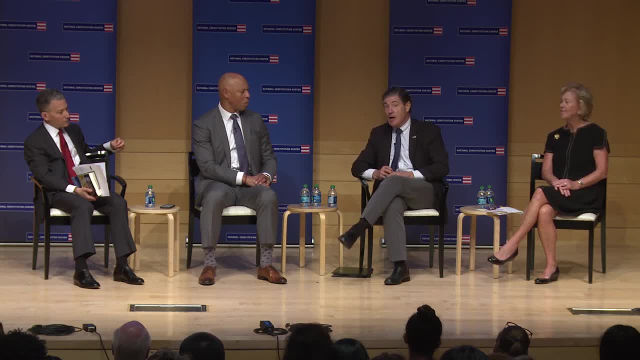 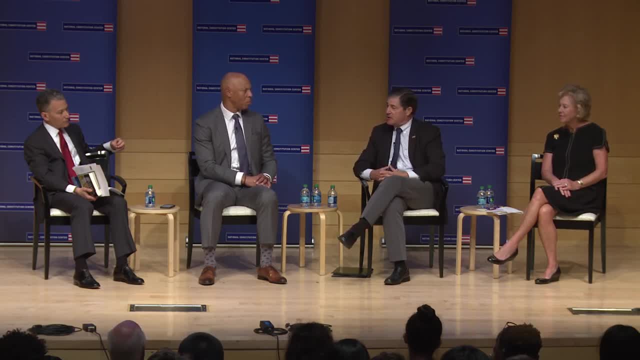 as members as well as other organizations, team together in what we call PA Civics to help with Act 35 implementation, to help add to the resources available to educators and to ultimately get into our communities again talk on a civil basis about our problems. 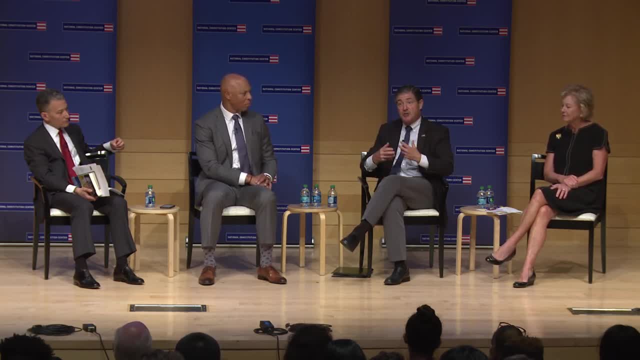 and how we can collectively have the skills and then ultimately undertake the action to deal with those problems. Thank you for that inspiring account of this really important act. It is wonderful that members of both parties have gathered together to support this nonpartisan requirement. 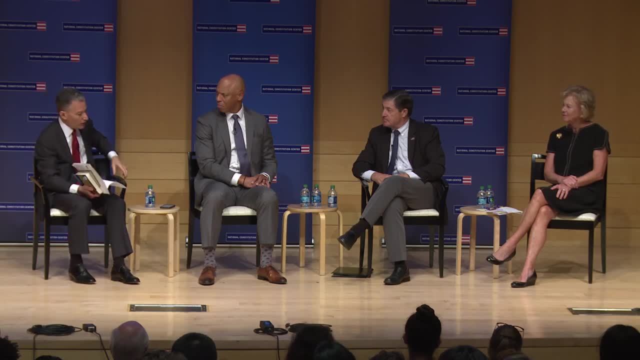 which, as you said, is necessary for good citizens to be formed and cultivated. And thanks for the work you're doing with the Civics Coalition and we're gonna look forward to working with you as well. Glad to have you. Great, Judge Rendell, you are a visionary leader. 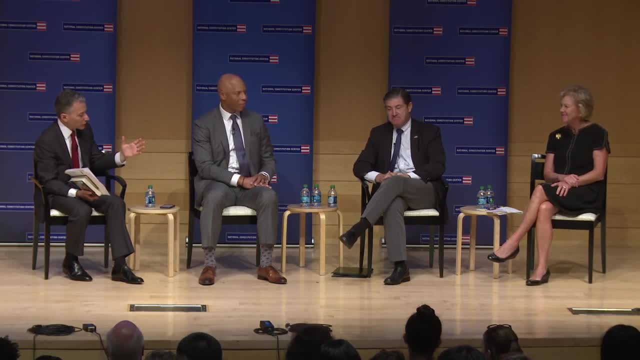 of civics education in America and your work at the Rendell Center and as an advocate for civics has galvanized people across the region and across the country. Tell us about the Rendell Center's latest efforts to promote civics and some of our exciting collaborations. 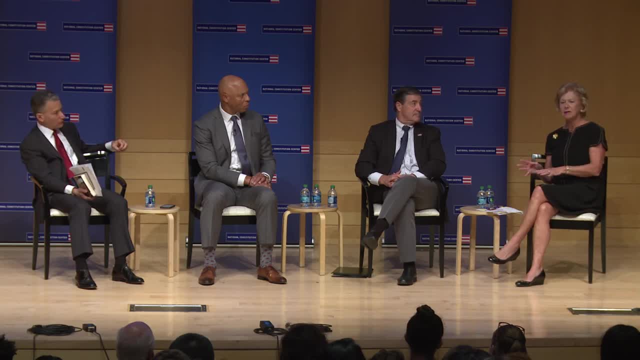 Sure, Thanks, Jeff, And actually I guess I'm wearing two hats here today. I am a federal judge and we deal with the Constitution all the time, And then I do chair the board of the Rendell Center for Civics. 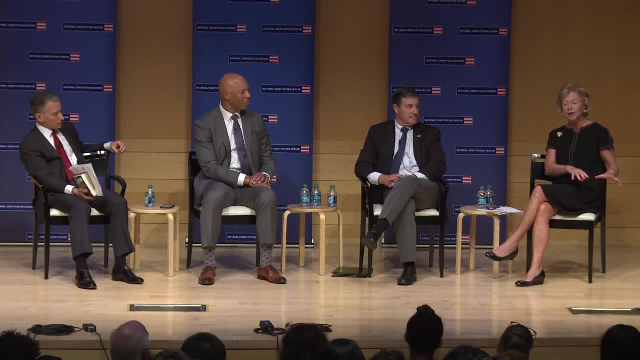 and Civic Engagement, which was founded as a nonprofit. about five years ago, After I left Harrisburg, I thought we needed to do something to increase the level of civics education in our schools, And the Rendell Center does a lot with our third, fourth, 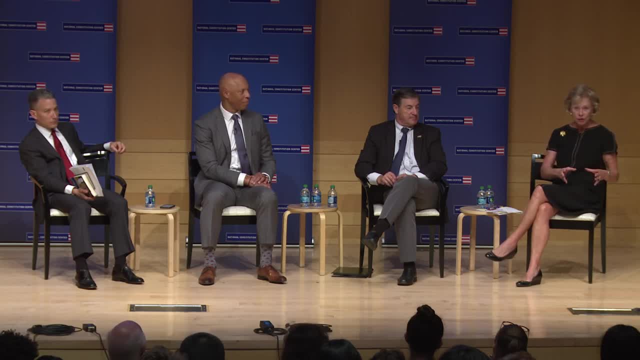 and fifth graders. We believe it's never too early to start teaching our children who they are. They learn early on about their community, their neighborhood, their faith, manners. So learning citizenship and who they are and where they fit really is possible at an early age. 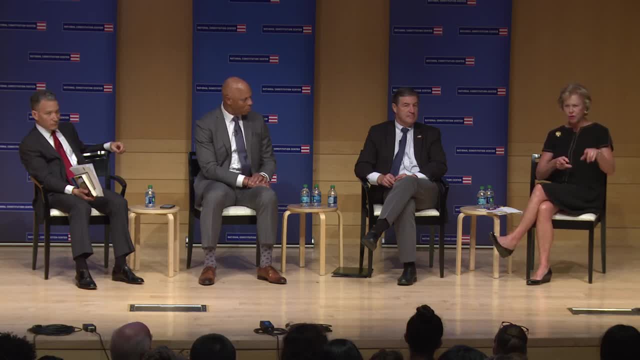 And it's amazing- Now I think a lot. we have a lot of middle school children here. I'm not sure, But it's amazing how in third, fourth, fifth grade they're like sponges. They really can absorb what we're teaching in civics education. 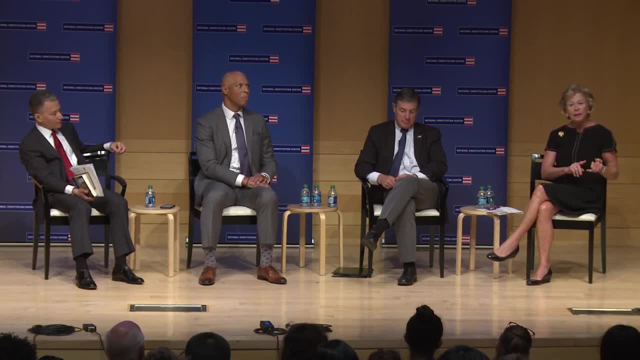 And so at the Rendell Center we have a few programs. One of them is called Literature-Based Mock Trial, And our curriculum director and actual lawyers go into a class and work with the literature that the students are reading, whether it's Monster or Hoots or whatever book it may be. 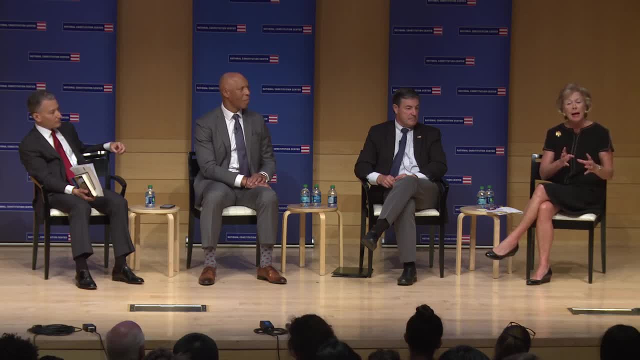 The students come up with. they pull a conflict out of the book and create a mock trial around it, And they create the trial, They have the witnesses, they put the opening statements, the questions, the closing statements And then they actually, when they're ready, put on the trial. 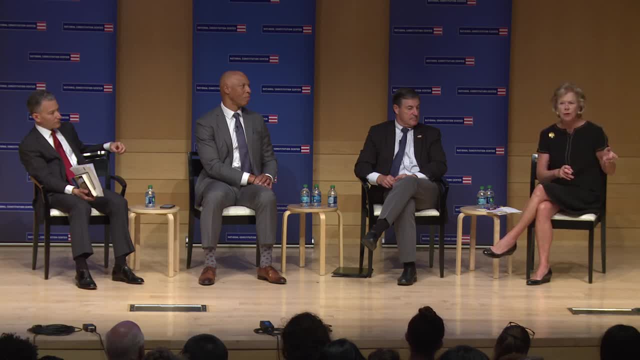 And very often they come to the federal courthouse. I think we had 22 classes had mock trials with an actual judge in the courthouse last year And I would encourage all of you- teachers are listening classes, all you students are listening- to get involved. 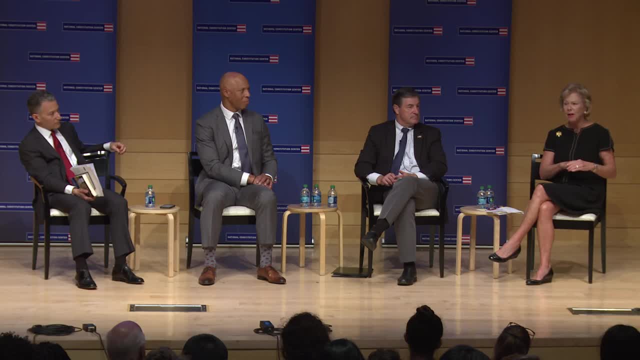 Contact us. We'll come in and help you put together a Literature-Based Mock Trial. It shows children how you know how to assess the judicial system. the importance of the jury Jury service is difficult for people But if you understand early on how important it is to have. 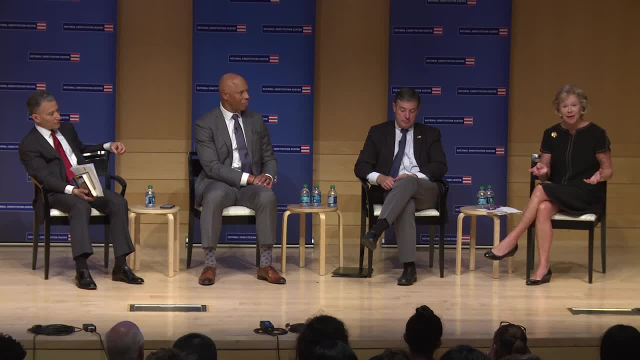 that jury and understand how to ask a question. a lot of what we do today in schools, I'm afraid, is memorization, But if you think about how am I going to ask this question and how am I going to make an opening statement, 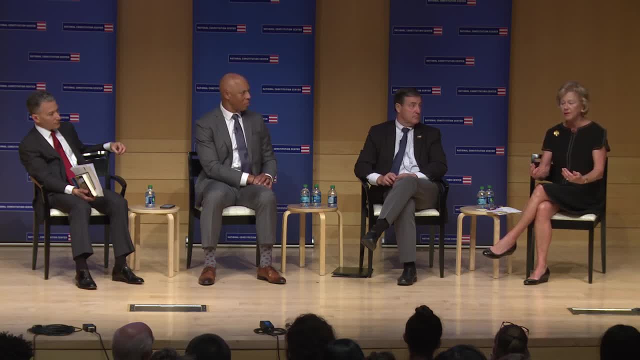 and letting children hear their voice in a really positive way. So that's one of our programs. Another one is called the Citizenship Challenge, And we do that in concert with the National Constitution Center. We have an essay contest where 4th and 5th grade classes come. 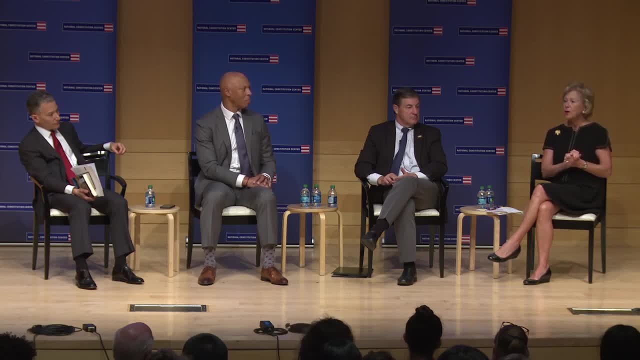 up with a response to our question Last year. the question was: what does the First Amendment mean to you? We get 250 essays from classes all over the region and we pick the top 10. We bring them into the National Constitution Center with their teachers, their parents. 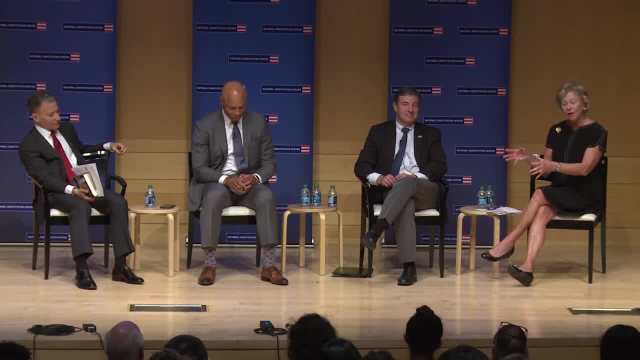 We fill the Kirby Auditorium twice And they have to put a skit on about their essay And we ask them questions Again, hearing their voice. They're not just parroting something, But they're really thinking about it And they research these issues and really find them not only educational. 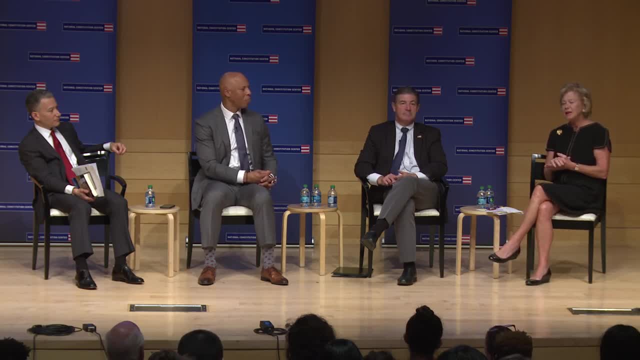 but also fun. The last thing we do is we have debates when there is an election And Governor Rendell loves this program. We had debates with Governor Wolf and his opponent. We had mayoral debates And we select five students from across the region. 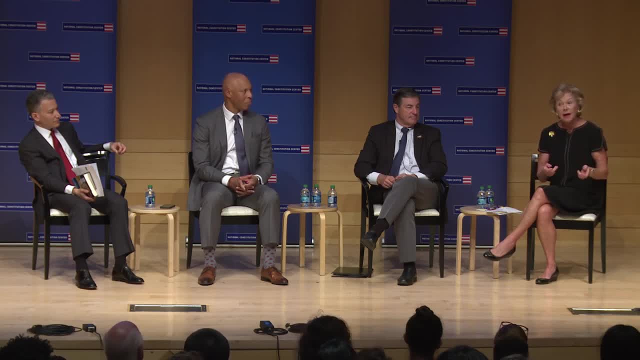 who have submitted questions they would like to ask And they come and the students ask the questions, Sometimes the tough questions- What can you do about crime in my neighborhood? And we get the answers from the candidates. So Governor Rendell is really a fan of that. 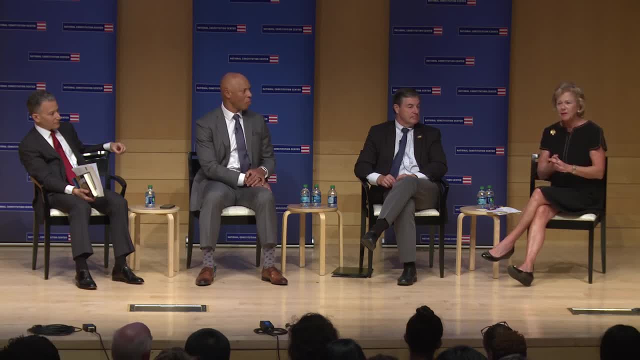 So that's kind of what we do from the Rendell Center, And I would like everyone to know that if you want a judge to come talk in your school or a lawyer to come talk in your school, we're only too happy to do it. 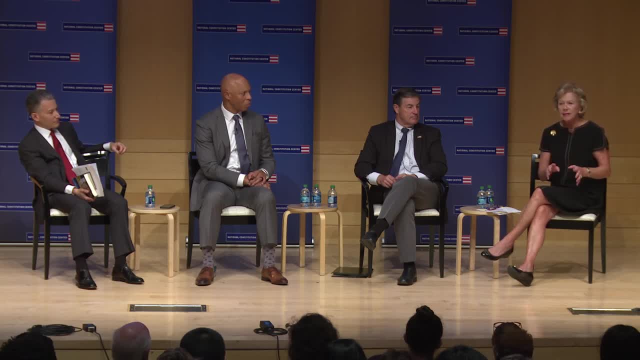 and to share our knowledge of the Constitution and civics and education. Thank you, Thank you, And we want to be a part of the discussion. We want to be a part of the discussion. We want to be a part of the discussion. 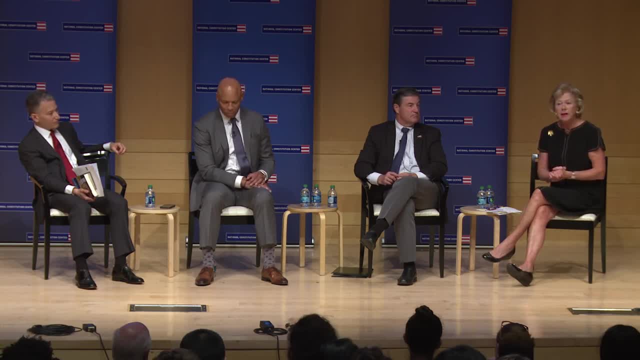 I want to be able to have a discussion with a judge and a judge who can educate you about the judicial system or whatever you want to hear, And people don't realize that that's possible, But we love going out and educating children, So just a little bit about as a judge. we have what's called a Courts and Community Committee. in the Third Circuit Court of Appeals, Which is in the Federal Courthouse right across the street, And we come to the National Constitution Center Whenever there's a class coming in we'll get a call and say: do you want to do a judge chat? 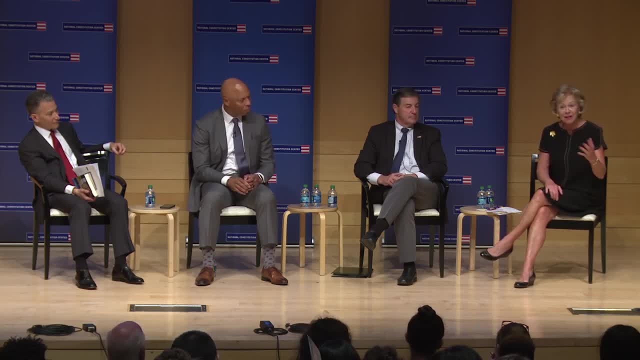 And we have a Court of Appeals And we have a Court of Appeals And we have a Court of Appeals and we have the coordinator of the courthouse who gets volunteers to come over. and I've come many times and we'll sit and tell the class. 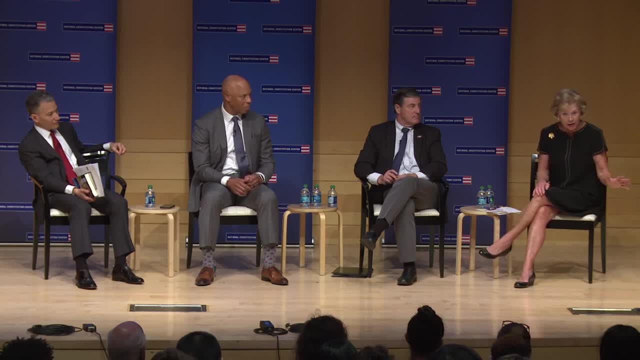 what we do and answer questions. I've been asked if I know Judge Judy, And I say no, I don't know Judge Judy, but I know Chief Justice Roberts and that's a little bit more important, if you know what I mean. 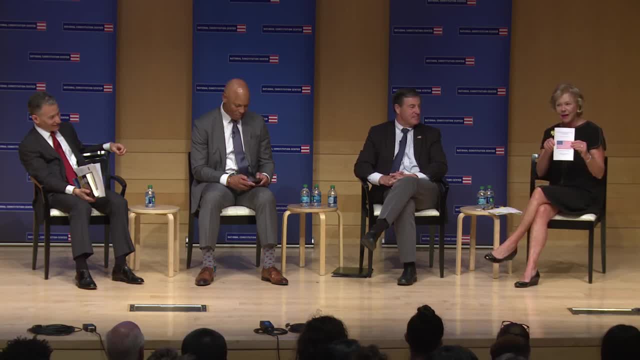 We also oversee naturalization ceremonies, and there was one that happened this morning. Judge John Padova oversaw a naturalization ceremony which I think there were about 40 new citizens from 25 countries, And to look out on the faces of these people. 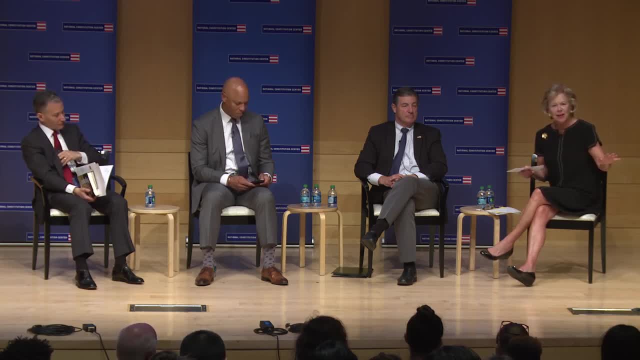 who have come from all over the world, leaving their homeland to come to this country. it doesn't happen anywhere else, It happens in the United States, And to hear them talk about how thrilled they are with becoming American citizens, it's a wonderful thing. 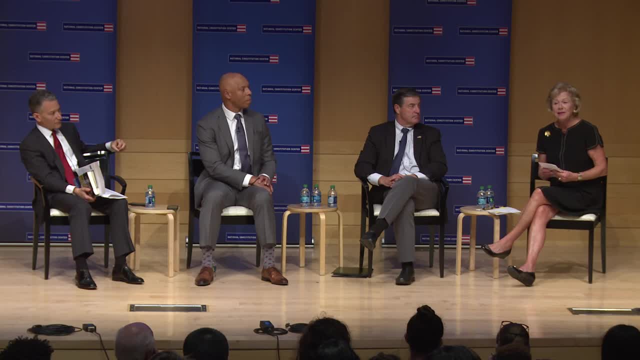 And now, with all the talk about immigration, it's really amazing that we have so many people who are working towards citizenship and working hard. They really want to become citizens and it's really an excellent program, So I would encourage teachers also to bring your students to see a naturalization ceremony. 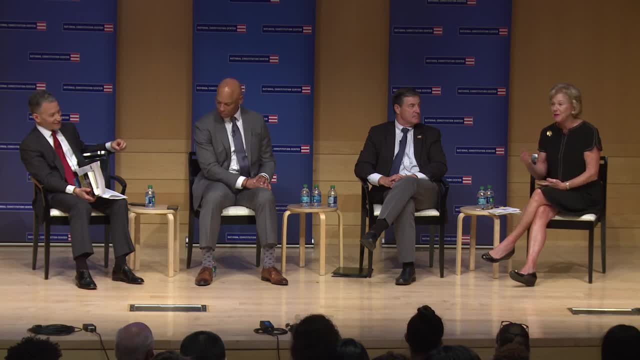 So all of these things, I think, although I'm a judge, I think the things I'm doing in civics have more impact, probably, than my day-to-day world. So it's enjoyable and it's fun to help the children learn. 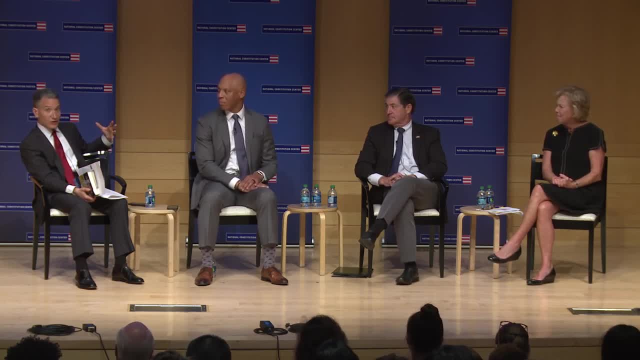 Wow, that's both an incredibly inspiring tribute to civics. And did you hear, Franz, what the judge just said? She thinks the work that she does to help educate people like you is even more important than the work she does as a judge. 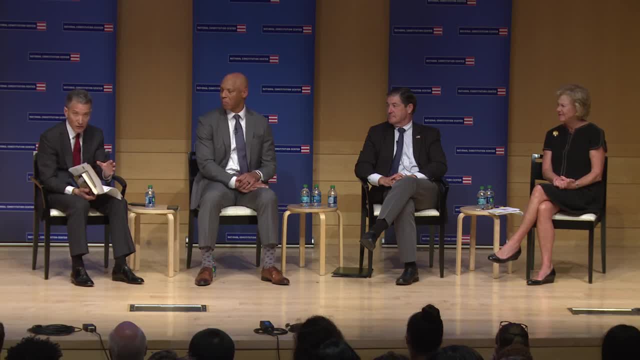 And you know how important that judge work is. deciding who goes to jail and who doesn't, deciding what our liberties are, That's very, very important for individuals, But I hear her saying that in the long term, having active, engaged citizens who 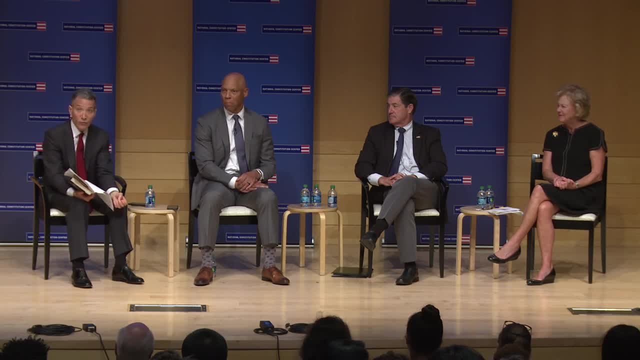 are able to be capable of self-government is even more important for the future, And I think that's why we're so grateful to you for learning And we're so honored to have all these incredible educators here to talk with. I have some questions for them about what. 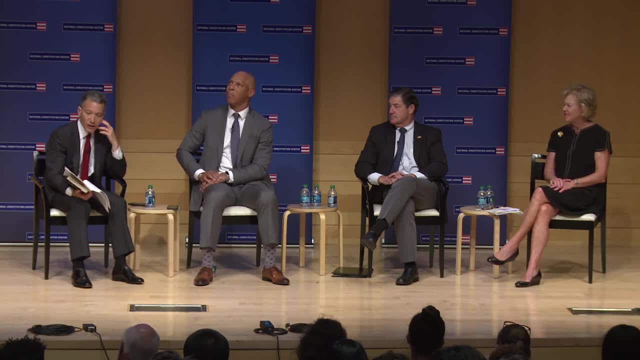 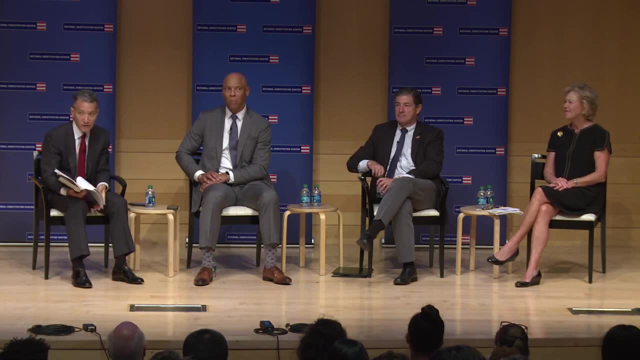 should be on the citizenship test and what we can help do. But we have just a bit of time for questions And if you have some, it's a great opportunity to ask any of these great leaders whatever's on your mind. So we have an open mic. 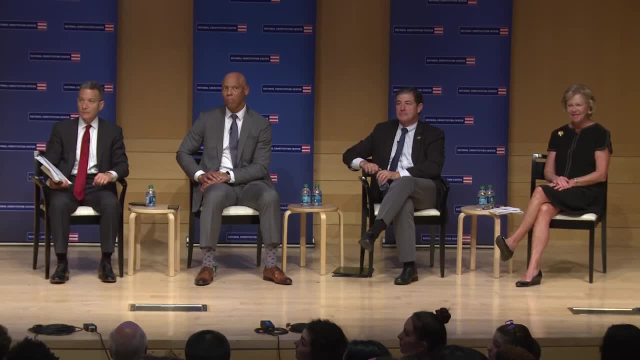 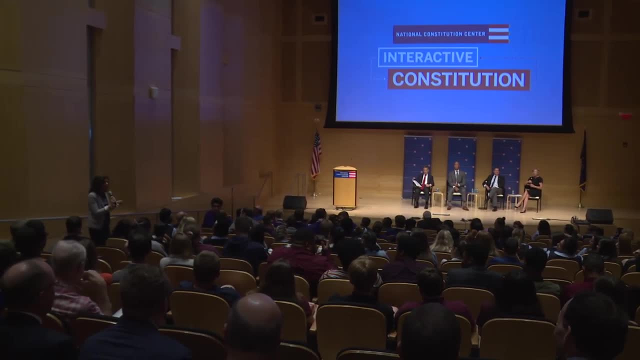 Does anyone have any questions for our panelists? So it's your turn and your time to have your voice heard. So, knowing the leadership that you have on that stage, what questions do you have about civic education in your schools And what things would you like to say? 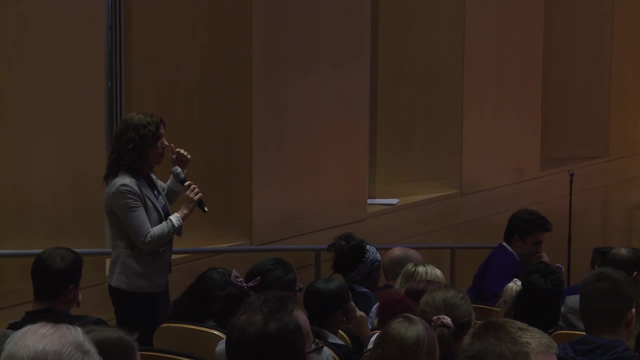 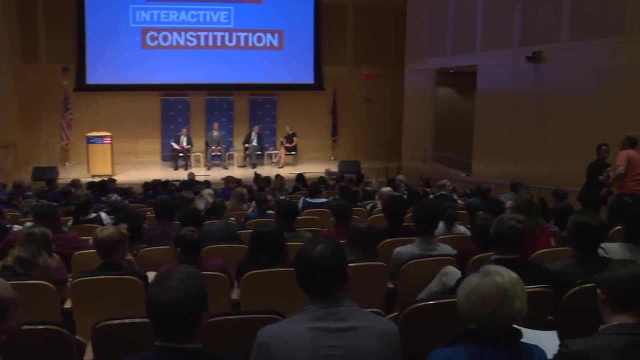 So if you'd like to ask a question, just raise your hand And we'll come over to you and get you started. Who wants to go first There? you go right over there. Oh, there's one, That was another student. 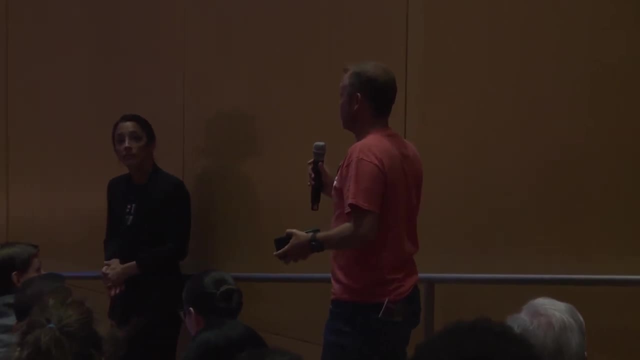 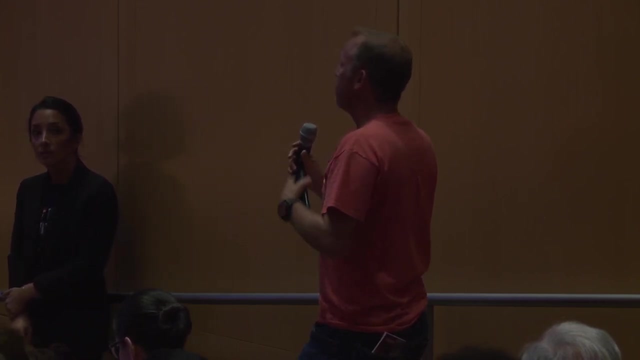 Good afternoon. Thank you for being here. I'm from Anchor Rancher Futures and we here in my school district we talk a lot about STEM and science, math, which are not really important, But when I sit down at my super intended meetings, 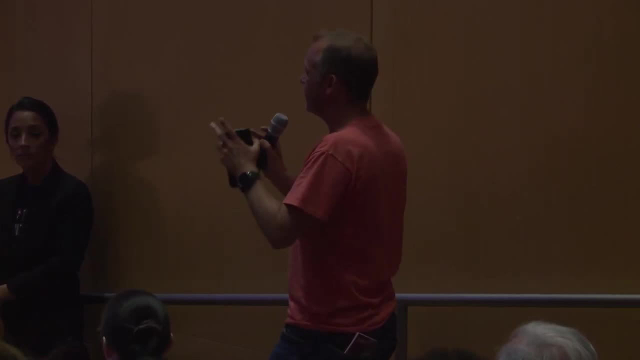 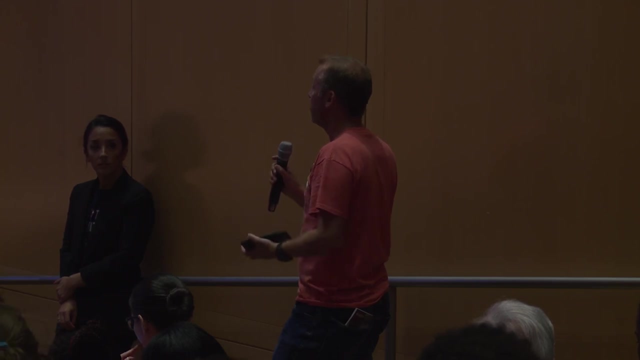 what would you make the case? How would you approach it? to say that civic education is important. I teach AP government politics so I'm getting those kids at the upper levels. But at the lower levels the kids are being pulled for all sorts of different activities. 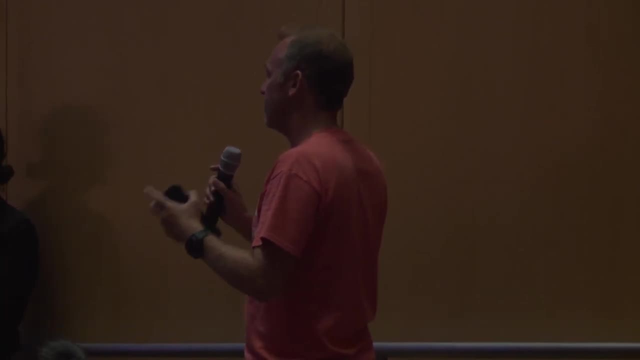 And we're not putting as big of an emphasis on civics and history and social studies as we should. So how would you approach it If you were in a meeting with my school and I was super intended someone who's more STEM-focused? 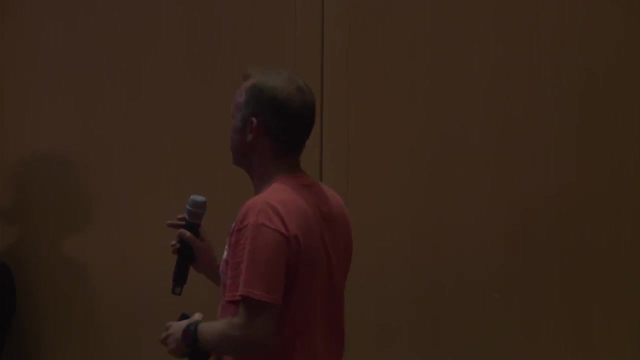 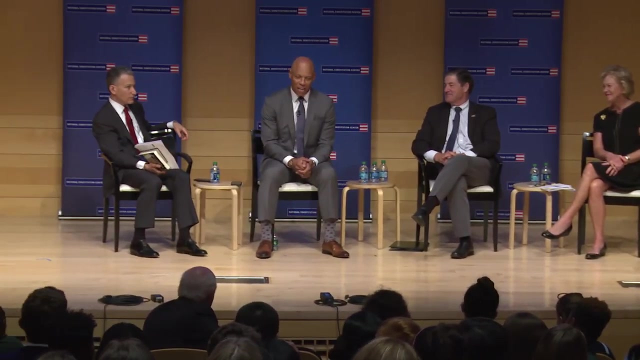 how could we make social studies and civics as well as STEM? What a great question. I think we should all take a crack at it. Yeah, so I'll start, because I would be likely to be in the meeting with your superintendent. 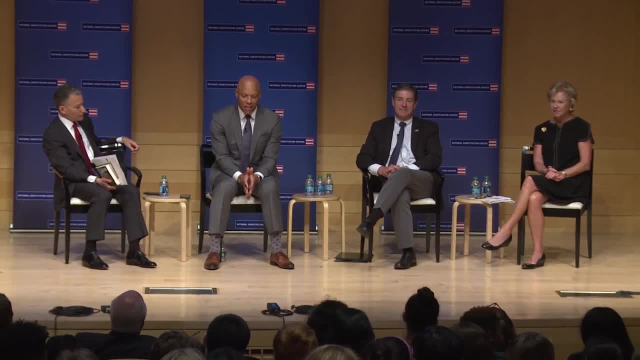 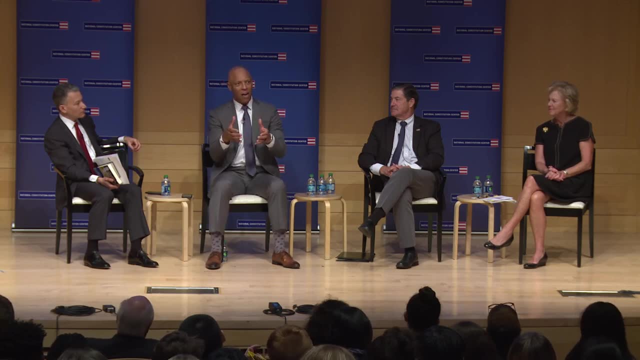 So one of the things that I think is really important is to not think about these things as mutually exclusive, And too often we silo content and then we are unable to draw any relationships with that content, And so there are ways to watch young people. 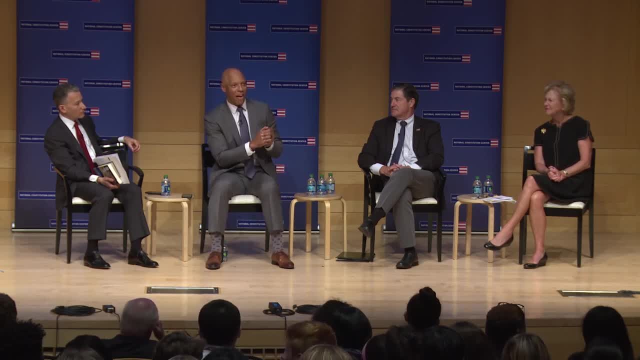 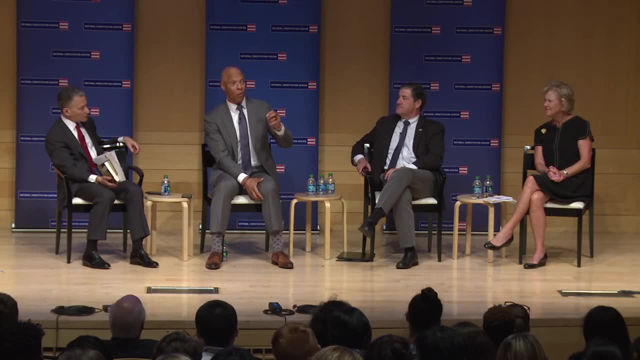 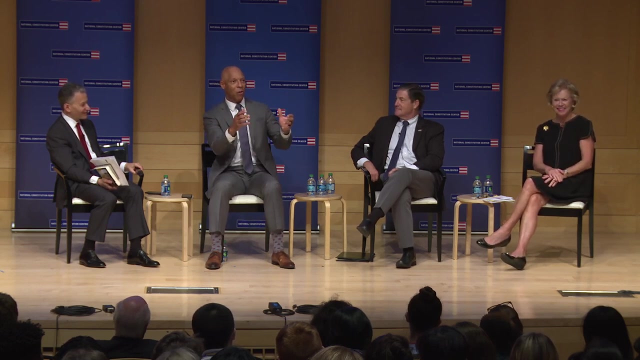 And Judge Rendell just reminded me of when I saw third graders in action at EM Stanton holding trial for Red Roddy's, the Fantastic Mr Fox. And so I saw the young people, I saw the judge, the jury, 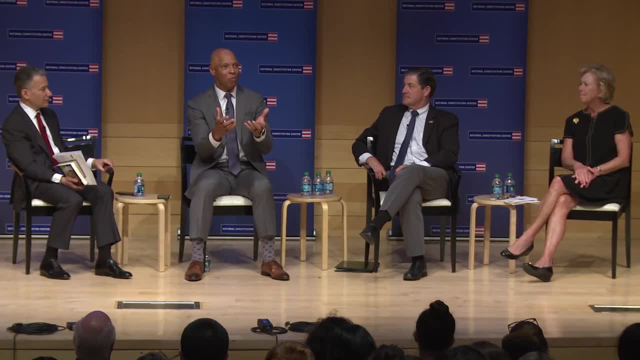 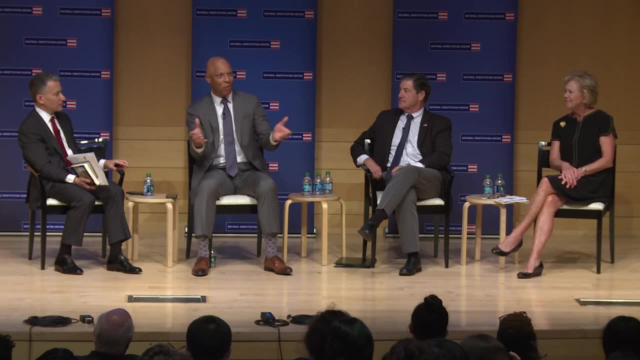 and then they actually had facts in which they had to consider for that that was somewhat outside of the civics area But nonetheless as a part of that process, was considered as a part of that, And so I think that, given where we are now, 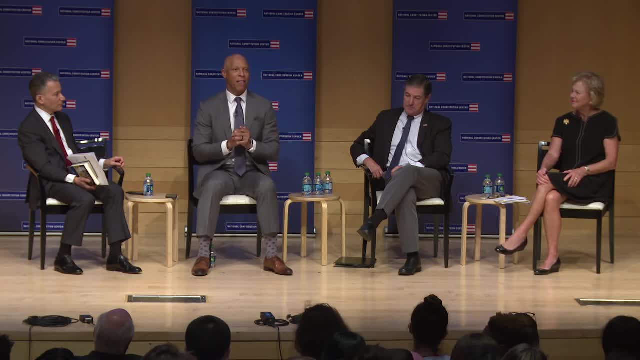 in terms of the conversations that's happening in our country, the conversations that are happening locally, the things that we need to do to inspire our young people to be engaged as citizens, particularly with voter registration and other types of things. I think there's nothing that's more important at this time. 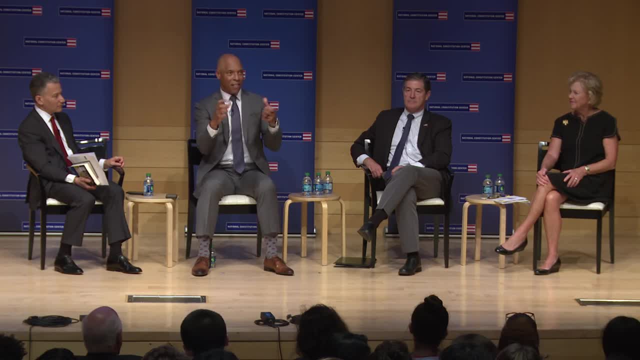 than to talk about how do we integrate civics as a part of that. And notice, as I was describing it, I wasn't saying the construction of civics as a standalone, but the construction of civics as a rewrite of content and materials that we already have in place. 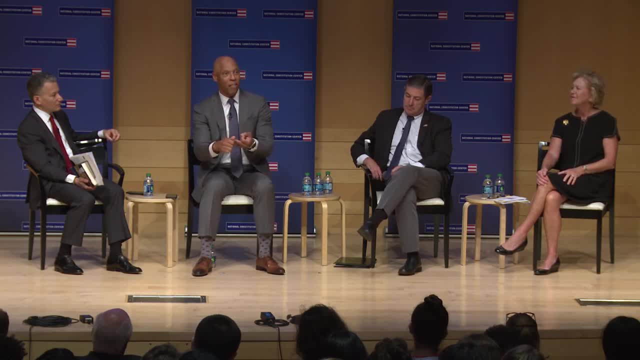 like US history, African-American history, world history. And then how does that become a part of that? And I think we have to continue to think about how do we make it a part and integrate it in a land, as opposed to a separate, standalone thing? 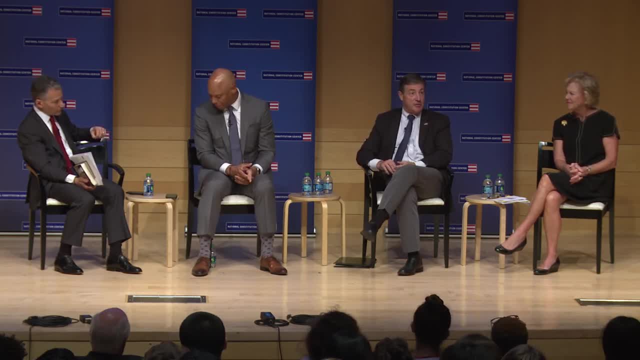 One of the things I found. I served in the state legislature for 12 years and then in Congress for 12 years, And I was constantly struck over that 24-year period about the number of citizens that didn't realize the power they had as a citizen. 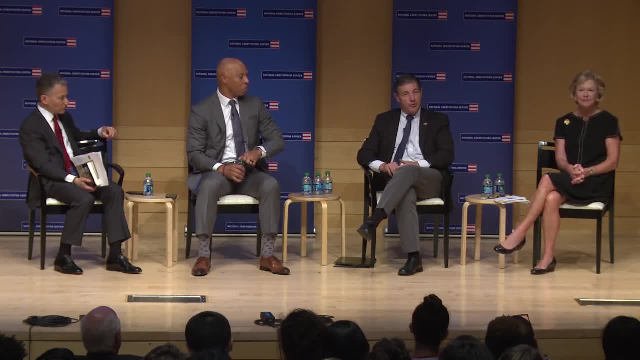 And so if you're in a state and you're a citizen and you're in school and you have a great STEM program, you're expecting your students who graduate from that program to go out and use the science, the technology, the math skills. 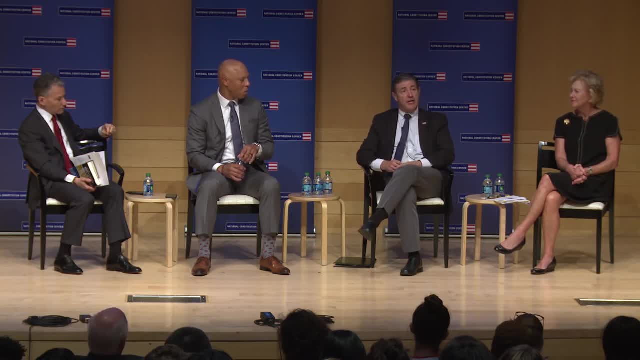 But we're having a lot of kids graduate from high school that don't have citizenship skills. So how can we expect them to exercise those rights and responsibilities if they don't have those skills once they leave school? And we want them to exercise those rights. 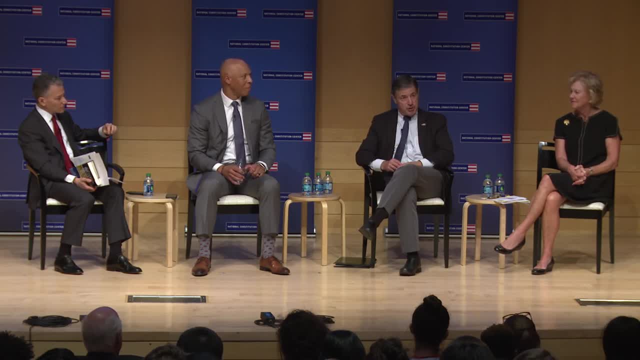 because they're going to have all kinds of problems in their community, in their state, of course, our nation And we're going to want them to have the skills that they need and we're going to want them to be actively engaged in finding solutions. 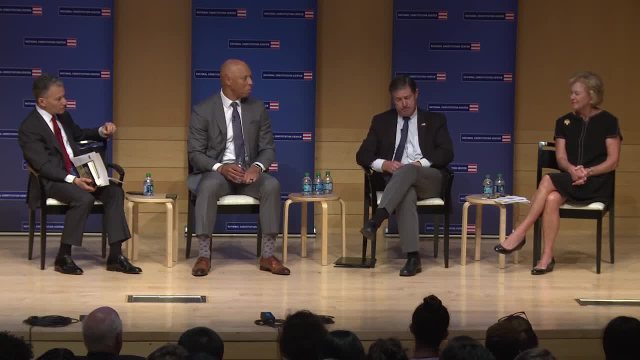 and finding common ground on a civil way or in a civil way, And so civic education is just as important as STEM, because you want them to use the skills they develop as a student to then use them when they leave school, And it doesn't matter if it's science, technology or math. 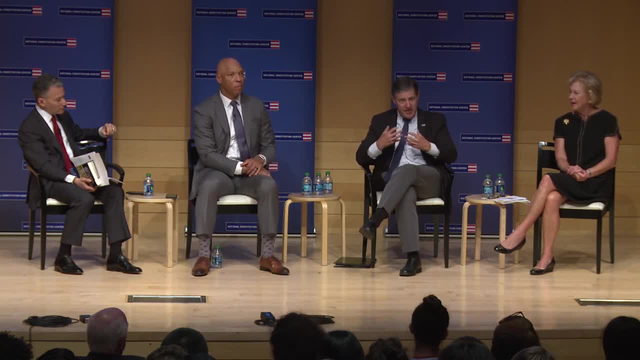 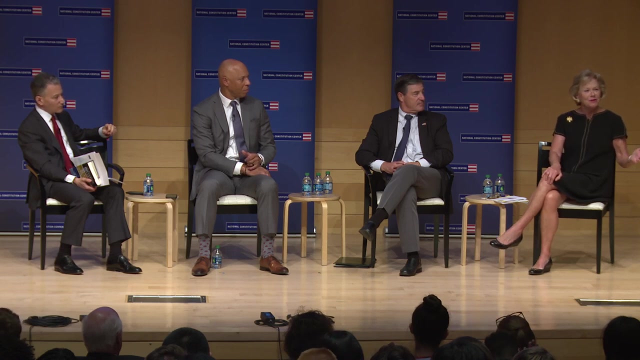 you want them to also be good citizens and to use those skills. That's how I would try to articulate it at your particular school meeting. And I would just add: I agree entirely with what's been said. but we're a democracy, But with the voting percentage now we're going backwards. 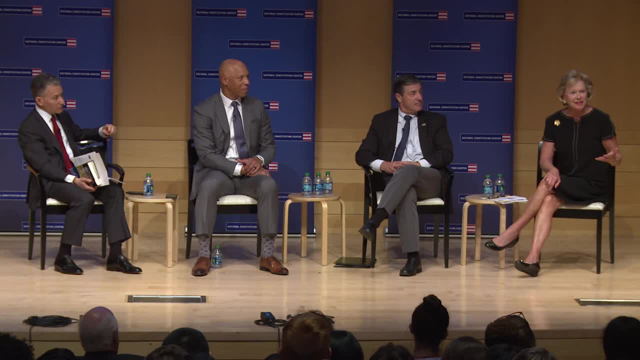 receding power to the few. People don't realize the power they have And the need we have as a country for everyone to speak and to vote and express their opinion. I think in the Obama election we were so pleased that so many 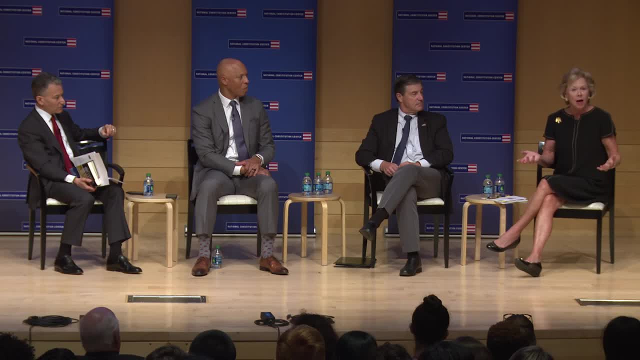 what percentage of our registered voters voted. You know, maybe 70% Unregistered voters. probably you know 25% of the population- Unregistered eligible voters voted. That's ridiculous. We're going back to the days when we were governed by a monarch. 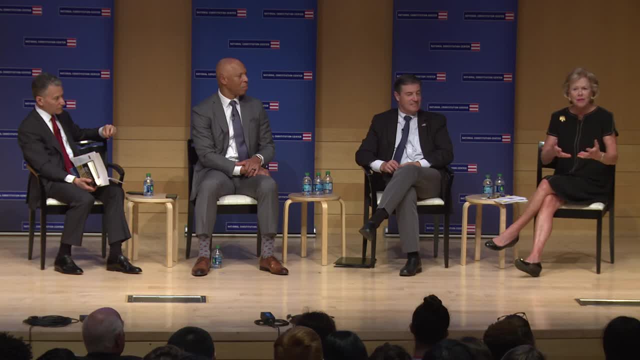 and you know you were kind of under his thumb. Well, we're under the thumb of the elected officials and we don't realize we have the power to do something about it. So I think it is and it's part of who we are. 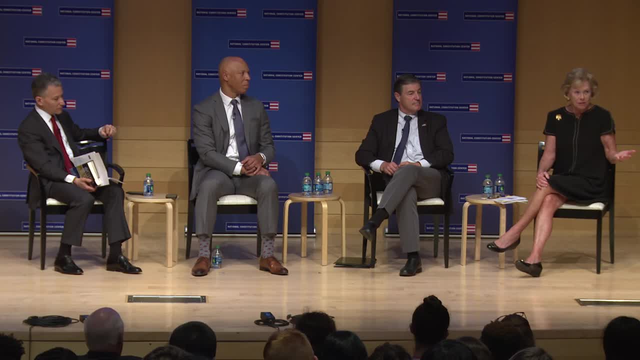 Our public education was founded on the principle of creating citizens, And our state constitutions all talk about creating good citizens. So our next generation- and that's why I say what I do with citizenship education is more important than what I do as a judge- because this is our next generation- 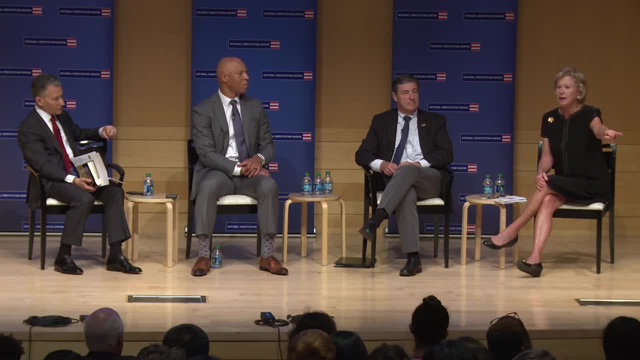 This is our democracy in action, hopefully in action If we teach them. it's important And I think when you put it on this macro level of this isn't a subject. it's who we are And you need to understand who you are. 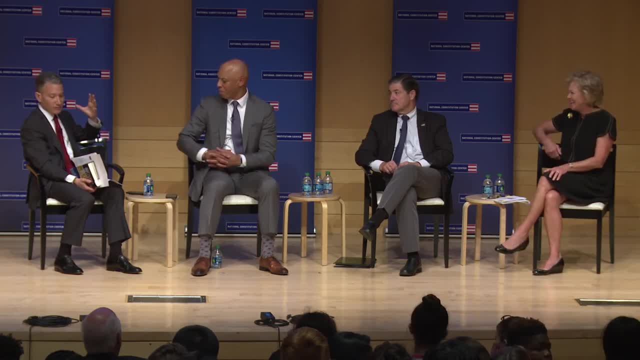 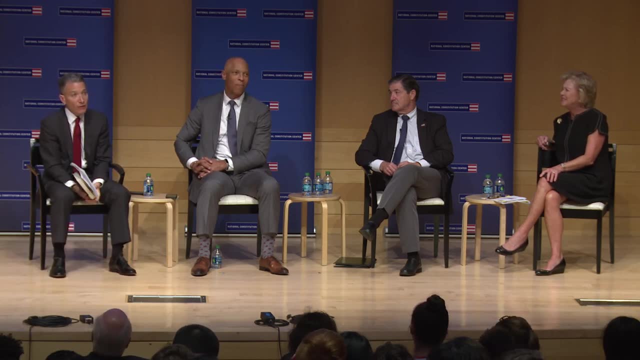 George, just if I could, just I can't resist noting that, George President Washington said that unless we educate citizens in the science of government, then the republic will falter. And Thomas Jefferson said that democracy cannot survive ignorant and free. We're seeing around the world young people embracing 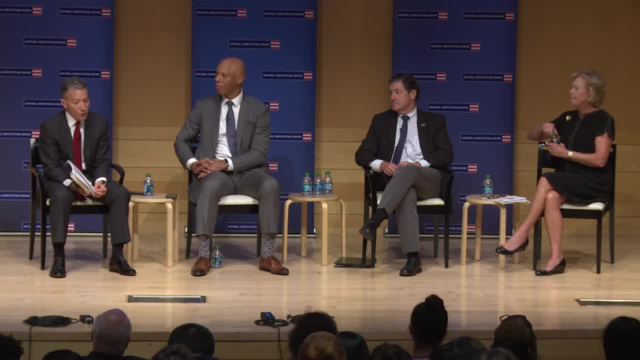 authoritarian alternatives to democracy, and those who are not educated in civics and the principles of constitutionalism are more likely to embrace these illiberal alternatives than those who are. So it's not an exaggeration to say the future of democracy depends on it. 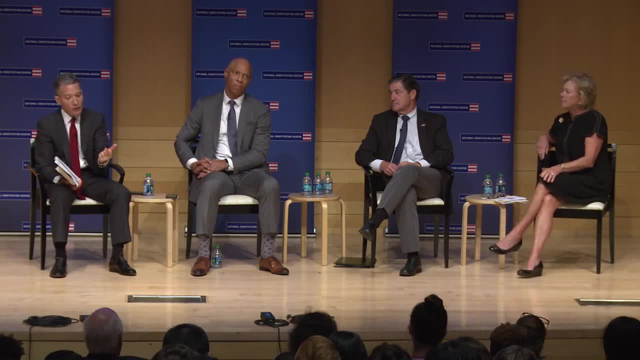 And that's why the College Board has decided to make two crucial requirements that it's aspiring all students to learn before they graduate from high school: code, computer code, that's the stem part, and the constitution. And today, on Constitution Day, the College Board 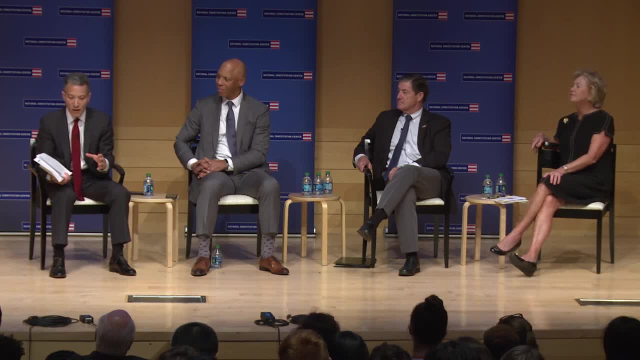 in just 15 minutes, right after this talk, is going to announce that they're encouraging teachers in all 50 states to sign up for our constitutional exchanges. We've already gotten teachers from 39 and they want all three to five million advanced placement students to learn. 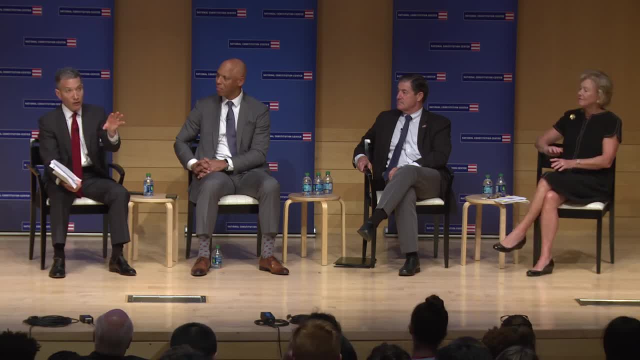 about the First Amendment on the Interactive Constitution, and then we want to bring it to non-AP classes and to students around the country. So we'd love for you to bring it to your AP kids and we'd love for all of you students to be part of this great effort as well. 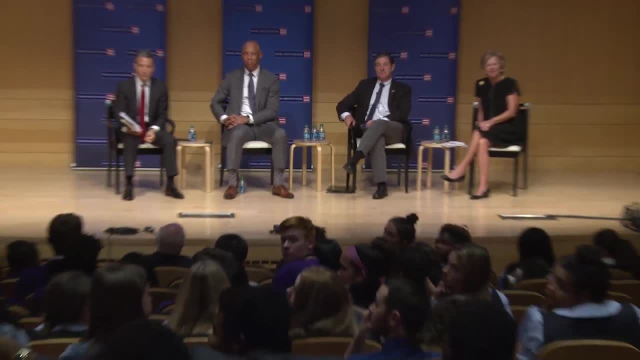 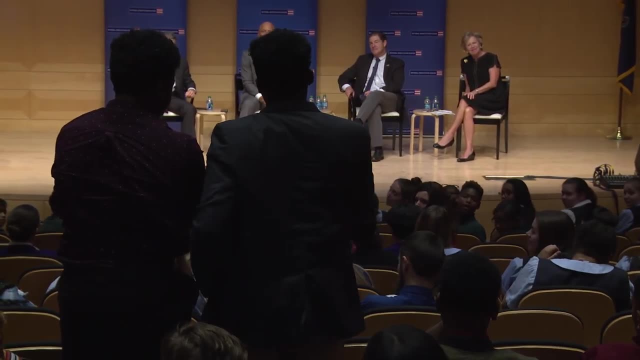 Great, Okay. question from the audience. Stand up, Gary. Hi, my name is Eli. I'm a student at the University of Michigan. I'm a student at the University of Michigan. I'm a student at the University of Michigan. 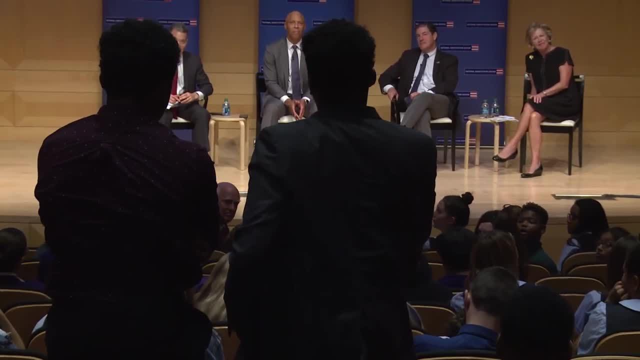 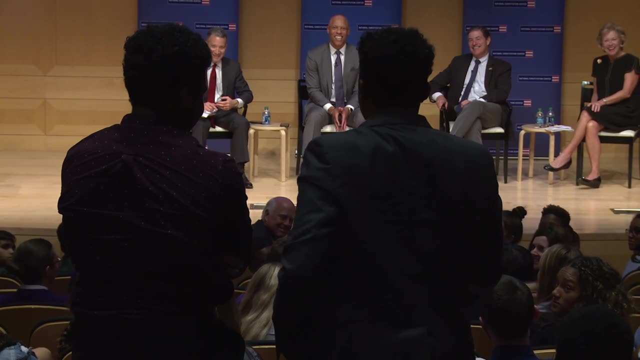 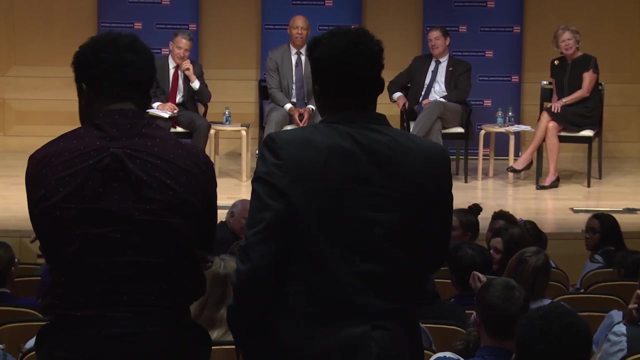 I'm 15 and I'm from Cal Poly School of the Arts in Wilmington, Delaware. This is my twin brother. He's been excluded, but my question is: as growing adults and soon to be the future of not only America but the world, which amendment do you think? 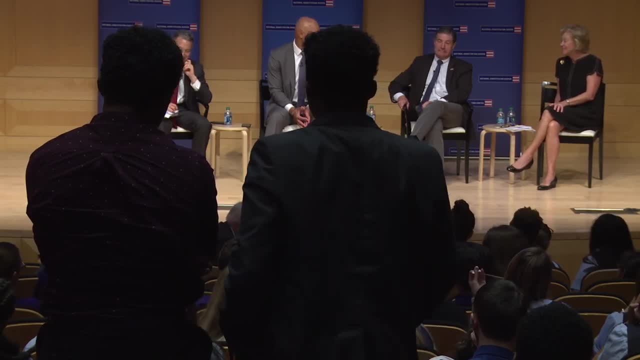 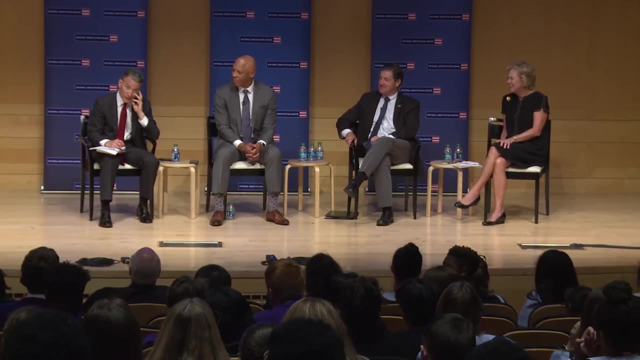 that we should hold close to our heart. Wow, that's such a great question. Yeah, good question. Wow, that's great. My boys are 13.. My boys are 13-year-old twins. They're just a little younger than you. 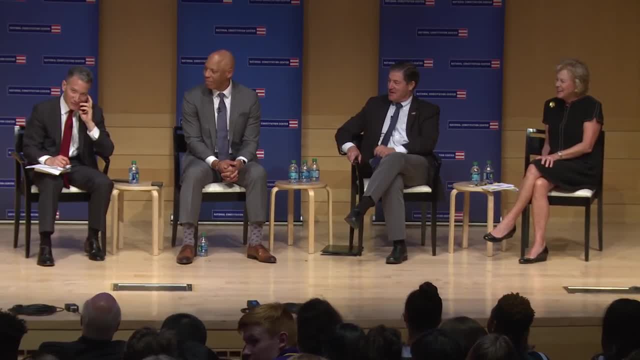 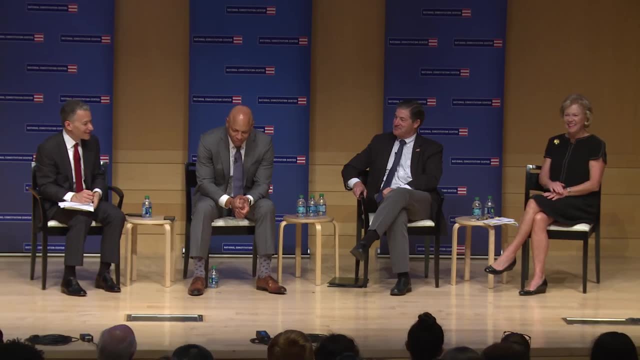 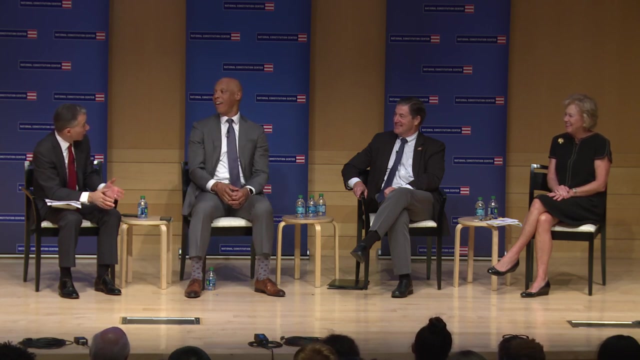 They're in public school in DC and they'd be proud of that great question. What do you think, Dr Hyde? Oh, you give it to me first. Yeah, It's a tough one. There are a lot of them, they're all important. 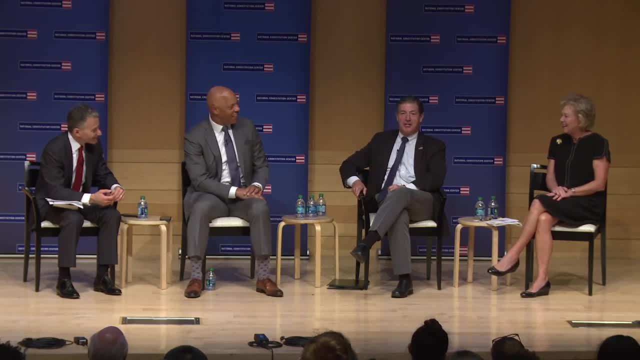 I would say all of them. How do you take any one of them and say, well, they're not as important, They're not as important as another. It was so hard to even get the Bill of Rights enacted. and then, of course, all the amendments that came from that. 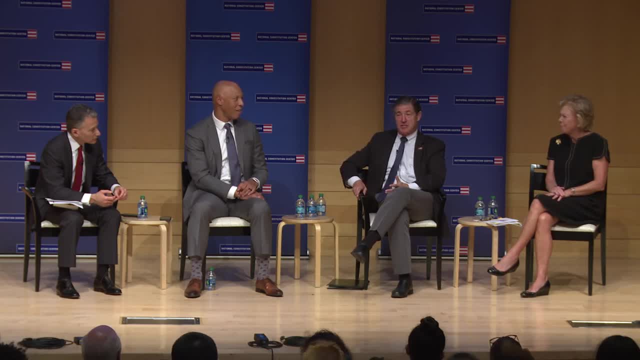 There's so few. ultimately, over 240 years of our existence as a republic, that even became an amendment to the Constitution. So they're all singularly important and they create this fabric of what we are now as a nation. So it's hard to just pick one out and say: 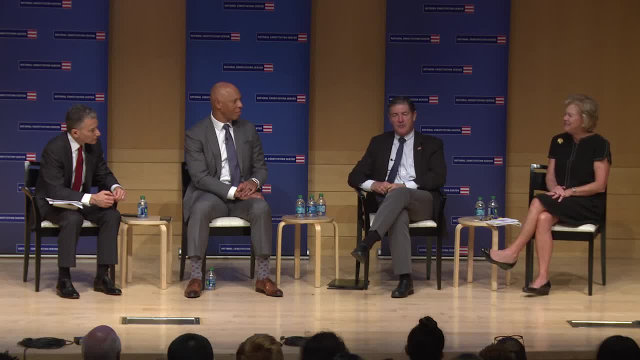 that's something I want to hold more dear to myself than another. They're all intrinsically important to who we are as a nation and there probably is going to be amendments down the road at some point. It's a really difficult process to get an amendment. 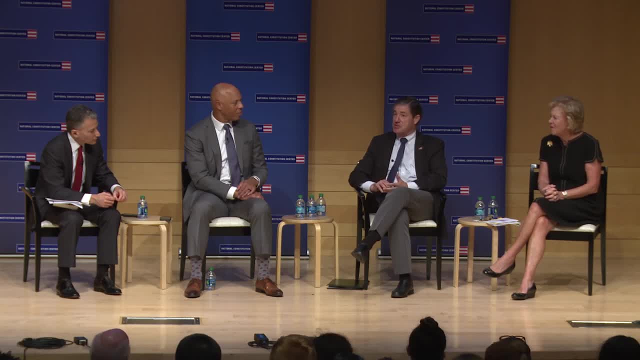 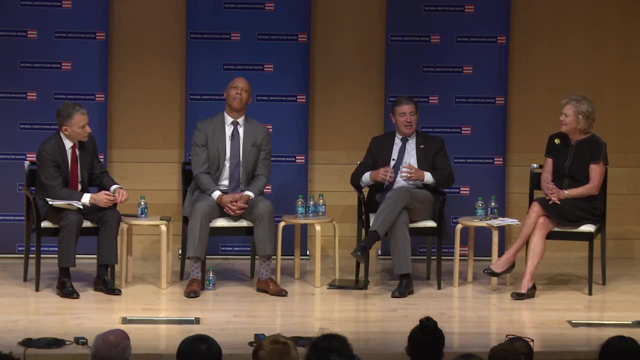 to the Constitution. but I wouldn't doubt our republic will go through some amendments down the road and they're going to be an intrinsic part of our nation at that point as well. So it's difficult to pull any one out, but maybe you have one Judge. 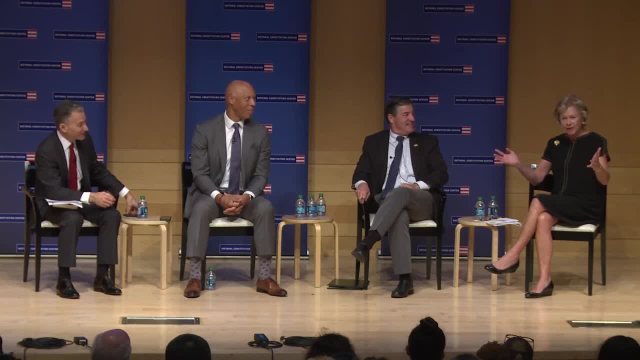 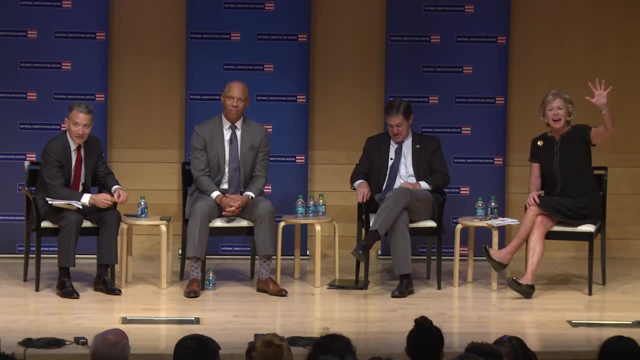 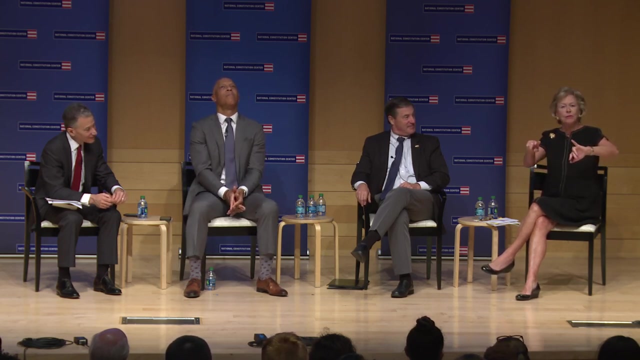 Well, I think the First Amendment came first. and how many freedoms are protected in the First Amendment Does anybody know? I see hands going like this Five. So just by sheer quantity we got press, religion, speech assembly, petition for grievances. 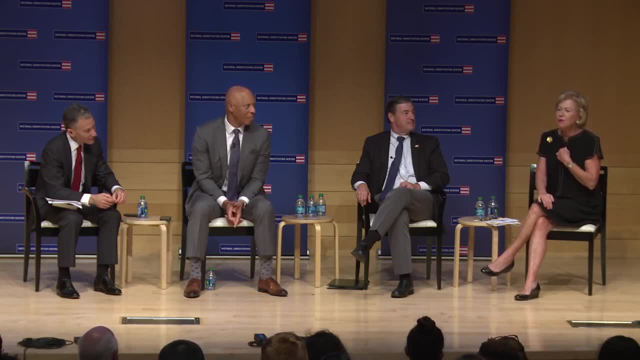 We got that's and that to me is a huge reaction again to what was happening in England and a huge reaction to the concept of censorship, and I just think that America, the whole idea of free speech and the whole idea of people being able to express their ideas, and maybe that's. 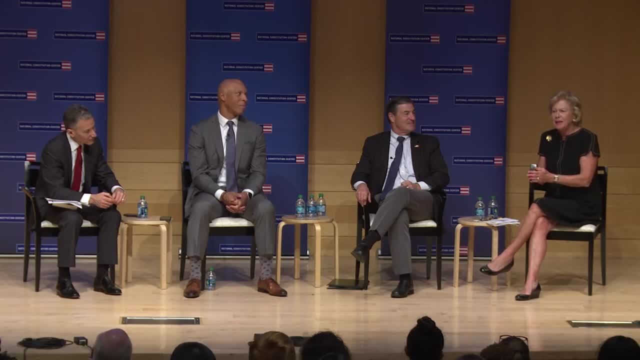 because I want the children to hear their voice. I think it's a really important one. The others are very specific. A lot of the Bill of Rights are very specific. you know: no quartering of soldiers without someone's consent, no excessive bail, no double jeopardy. 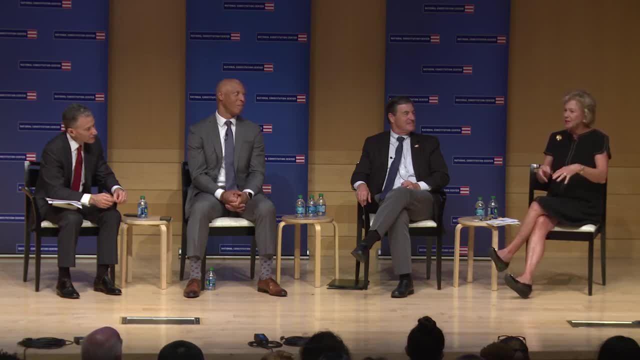 no taking of property without compensation. A lot of them speak to very specific things. I just think the First Amendment in its ideological scope is really- it's right up there- Very inspiring, Wonderful. Okay, he's ready. the other twin's ready. 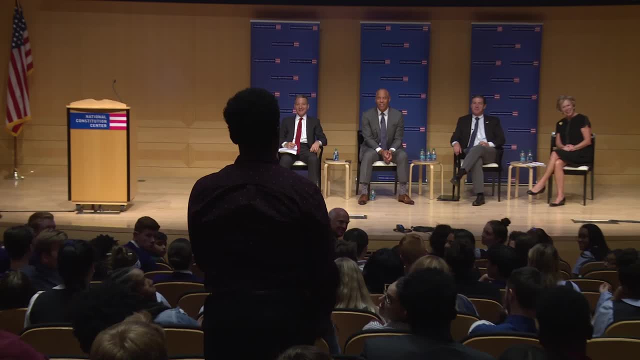 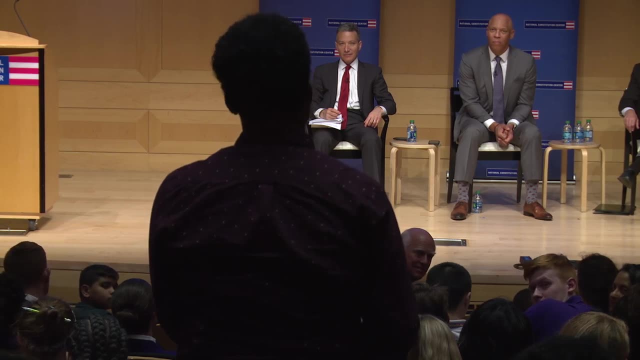 Oh good. Hi, my name's Michael Ruff, I'm 15, I'm 10 in Charlottesville, Wilmington. I'm also a member of the Wilmington Leadership Commission. My question is: somebody who is intrigued in the field of social studies and civics and wanting to do it as a career. 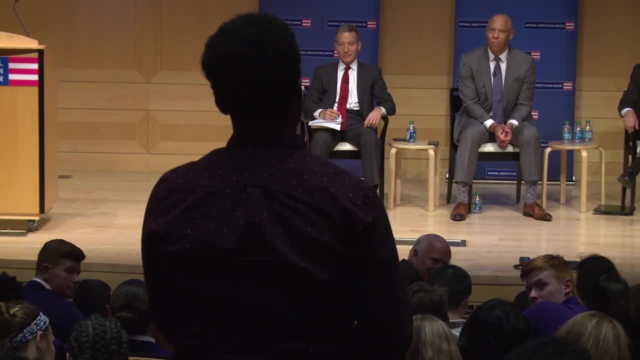 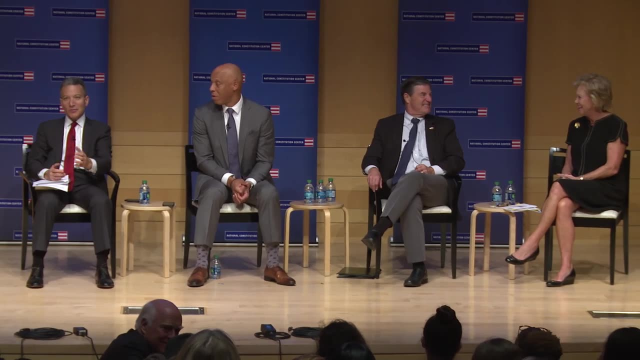 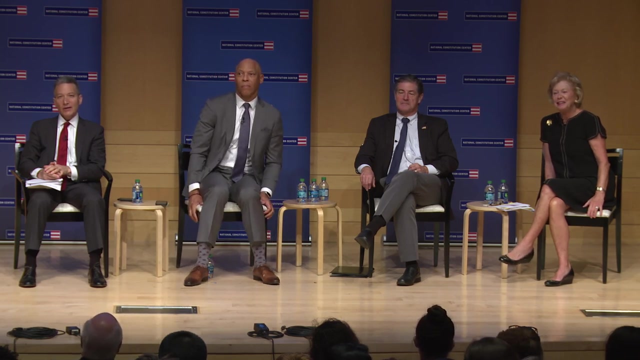 what tips do you have or philosophies or doctrines do you follow? Maybe an educated person? It's such an important question. The place to start is just to start educating yourself. read and learn as much as you can. It's so exciting the way one book can open up ideas. 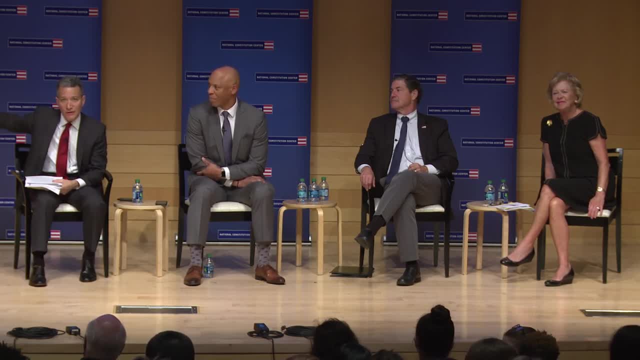 to something else and I just I think, if you just go to this website, constitutioncenterorg- interactive constitution, pick an amendment you don't know about, maybe not even the most important one, like the first, but pick something like the third. 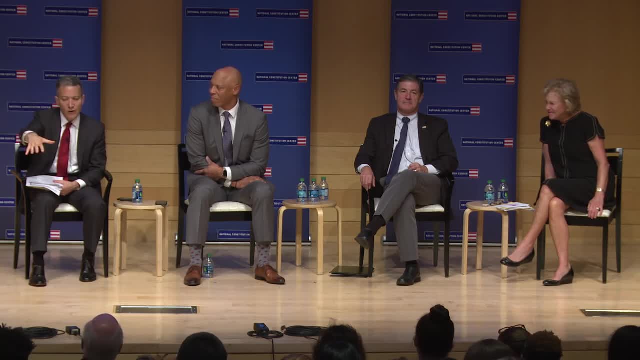 which is sort of unexpected. Why did the framers want to prevent soldiers from being quartered in the home? What does that say today about the fear that the government could intervene? Why did it invade our homes? And then you learn about history and you learn about text. 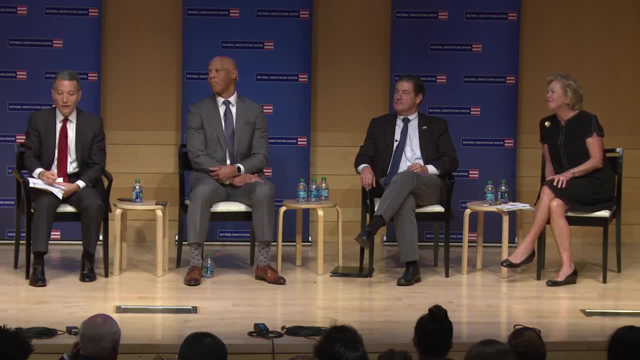 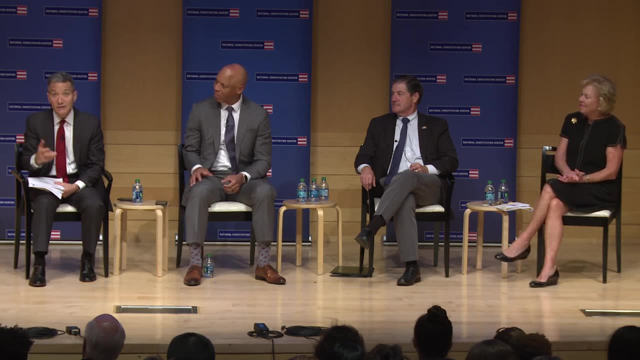 and you start browsing and learning and it can just lead to all sorts of unexpected places. I'll just say very quickly that when I graduated from college I went to law school because I didn't really know what to do. I knew I loved government and I loved English. 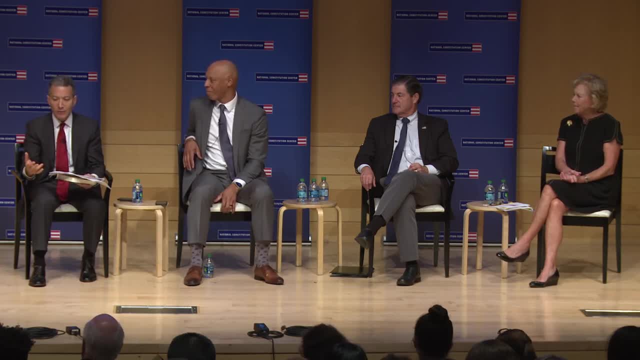 I loved writing and reading and learning about government but didn't know what to do for a living. And I just so fell in love with the Constitution in law school and decided to be a journalist to write about it and then a teacher to teach it. 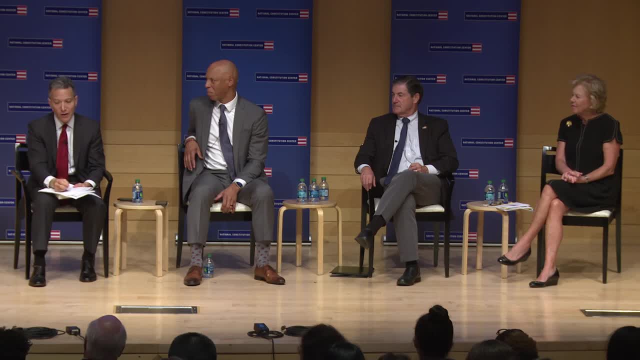 And you kind of just follow your calling by doing something that you love and are driven to learn as much about. So spend as much time of the day as you can, not just reading for school and trying to pass the test, but reading because you love it and are interested in the material. 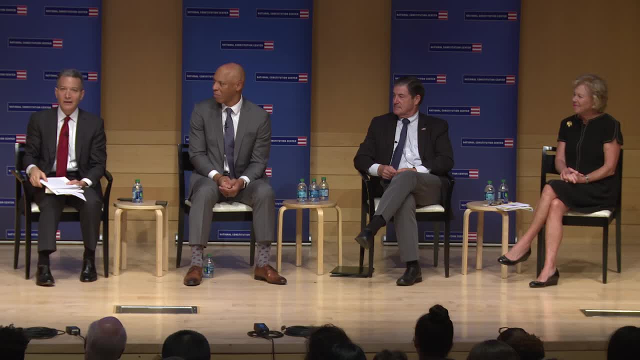 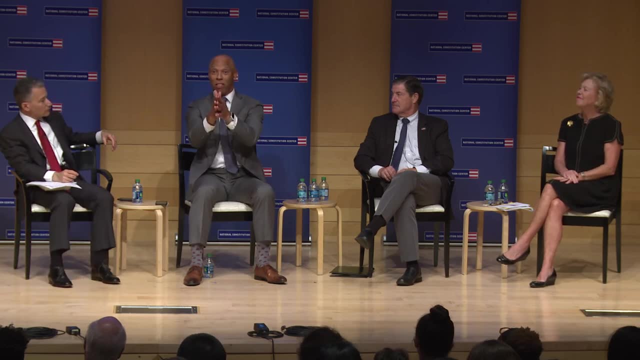 And if it's history and social studies, there's so much to learn every day. It's just a really, really exciting opportunity, If I may add, and if the young man wants to be a teacher, you're hired. So that's an important point. 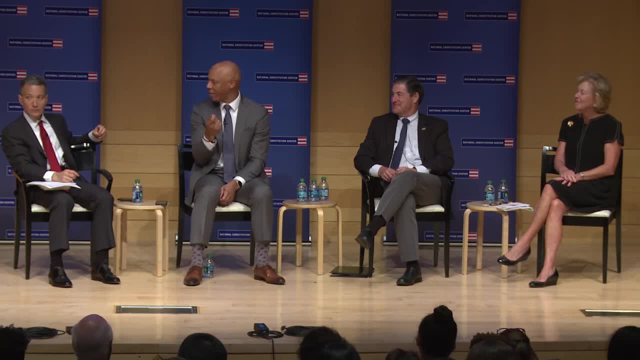 That's important And because I do think that one thing that is extremely important and it goes back to the other question about which ones do you hold close? and I was vacillating from the first the preamble, and thinking about this notion of student voice. 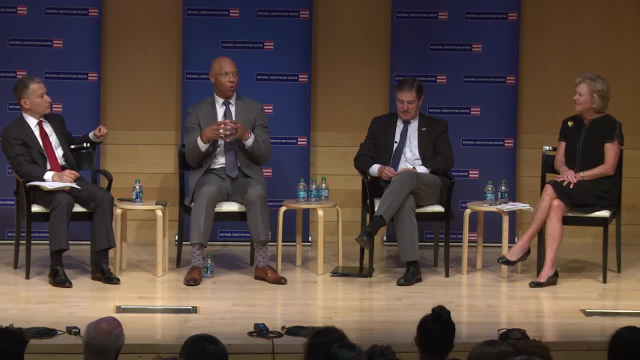 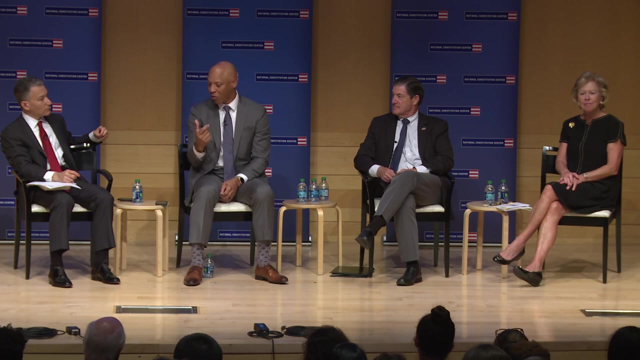 and the importance of us, as educators, to ensure that their voices are heard, and making sure that they have the knowledge in order to make their voices heard. So that's why I was thinking about the importance of the young man who just asked the question, if, in fact, he's interested. 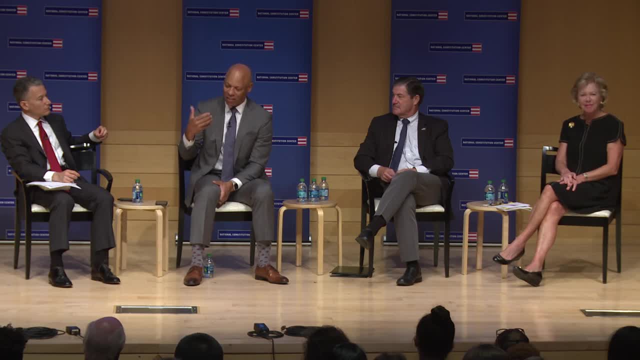 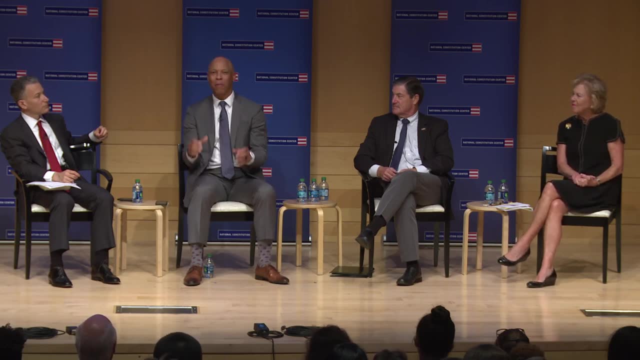 in the Constitution and civics, then the other thing that you should consider is then: how do you share that knowledge with other individuals? and think about that as an educator, moving forward as well. Just putting in the plug, Bravo, That's so important. 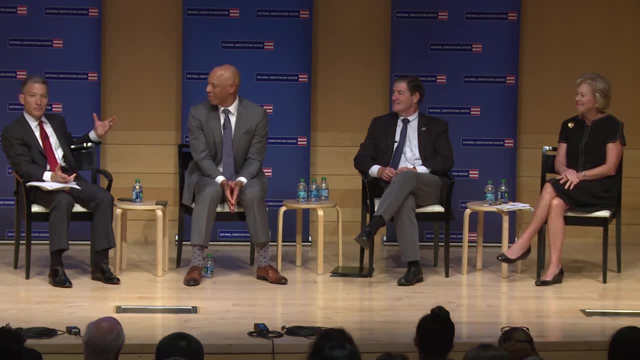 There's nothing more fulfilling than being a teacher. To be a learner is to be able to be a teacher, and you teach in the course of learning more and more yourself. I think we've. I'll just throw one extra one in. Just pick out one problem in your community. 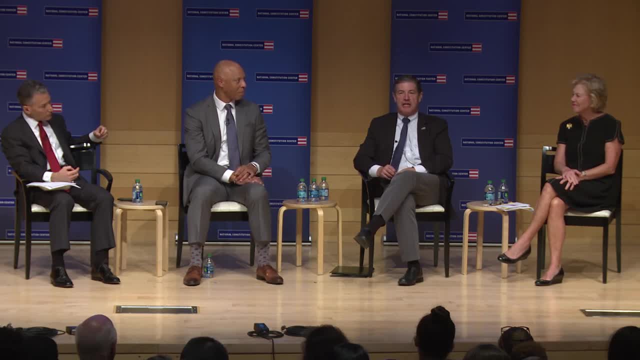 Do all the reading, educate yourself as much as you can, on as many subjects as you can, but also try to apply that knowledge somehow to problem solving. So what is a community problem that you're having where you live? And therefore, once I know what that problem is, 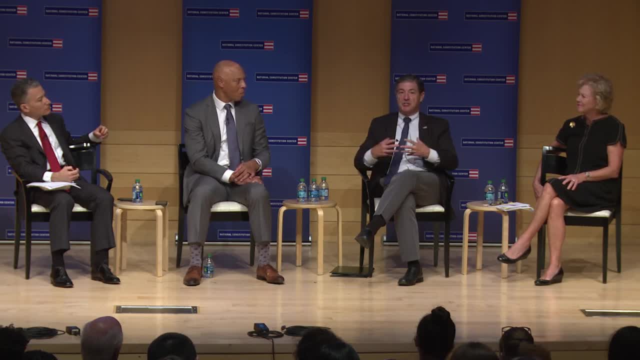 who can help me solve that problem. Who else do I need? I need to bring in to the discussion to find the solutions. Once we decide what the solution is, how do we then generate a group of people that want to work on that same solution to actually accomplish it? 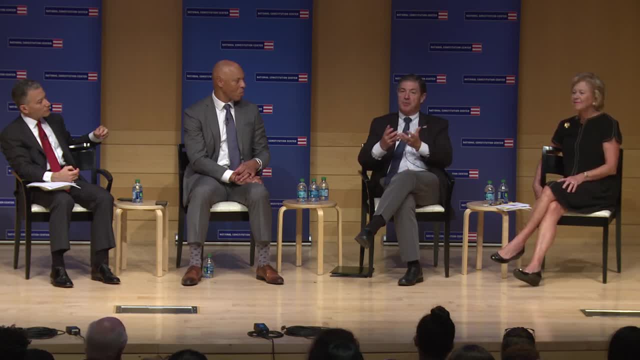 and to implement it. So it's taking that book, learning and applying it to real world problems that people around you have and then accomplishing something to move the community forward. That would be very educational. Something I found interesting along the lines of what Jeff was talking. 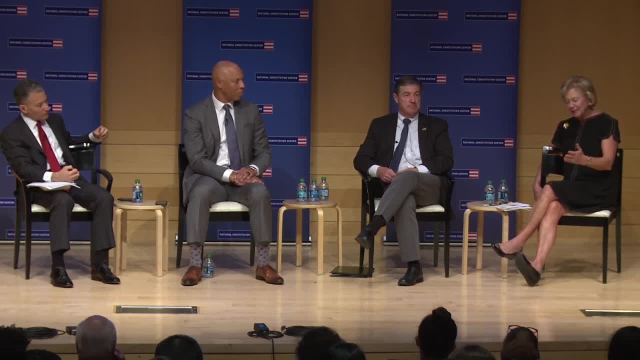 about, about reading and educating yourself. especially appropriate on Constitution Day is that James Madison, who's called the father of the Constitution, really came up with the idea for the structure and the balance of power, the checks and balances. the different we should have, the different branches- judicial. 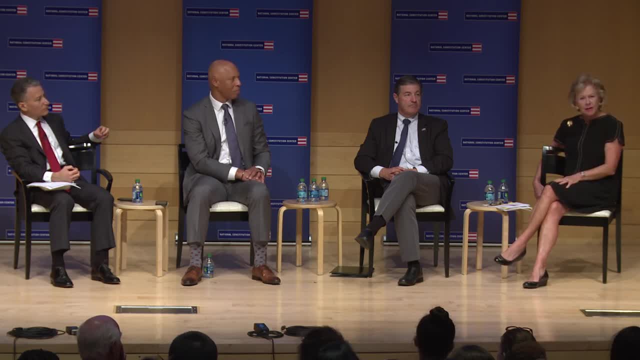 legislative and executive, And he just didn't make this up. Thomas Jefferson sent him a crate of 200 books from France. They corresponded And they were great friends. Jefferson was, I think, eight years older, But he sent him a crate of books on political science, on philosophy. 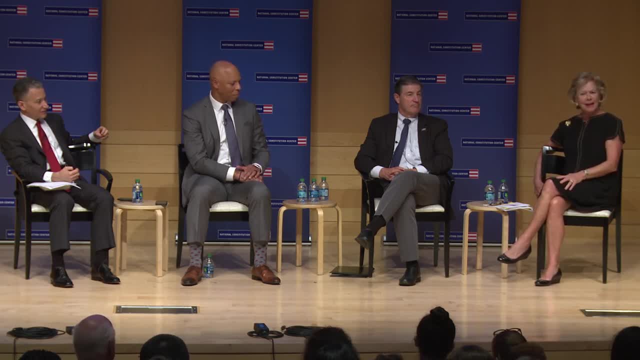 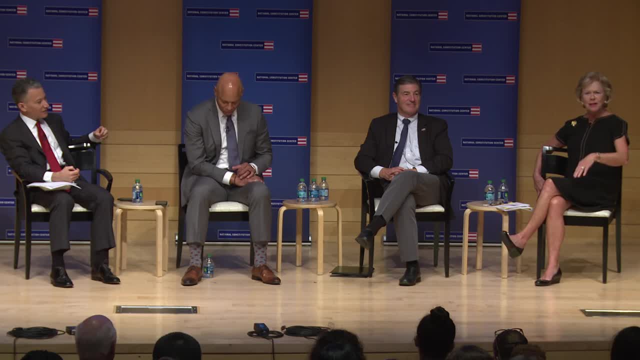 What books there are out there. You can get audio books You can get. you can stop reading them if you're not interested in it. I mean, there's just such a wealth of information now There's almost no excuse for for not turning to these resources. 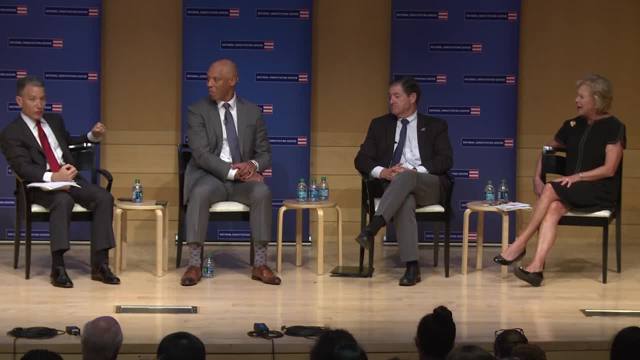 That is the perfect note on which to end, And we do have to end because there's another program that's about to come in. Think about the opportunity you have every day to read and learn. As the judge said, the entire world's library is at your fingertips. 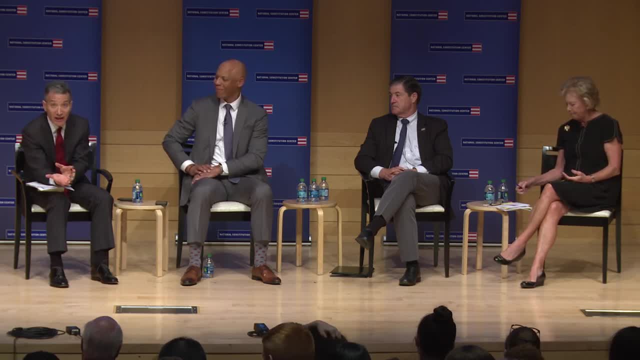 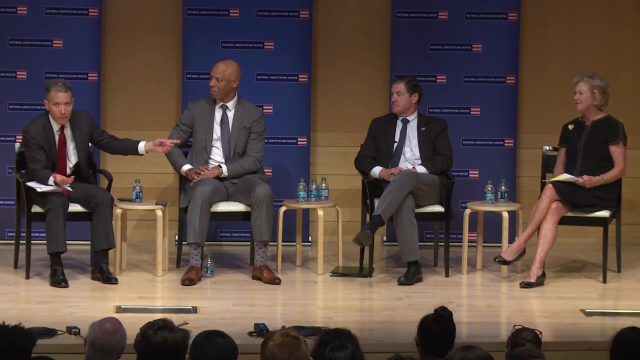 Incredible resources like that interactive constitution, the ability to get like any book from almost any time in history just by clicking. All you need is the discipline to read seriously and deeply to resist the temptation that we all have. that I face and I know all.